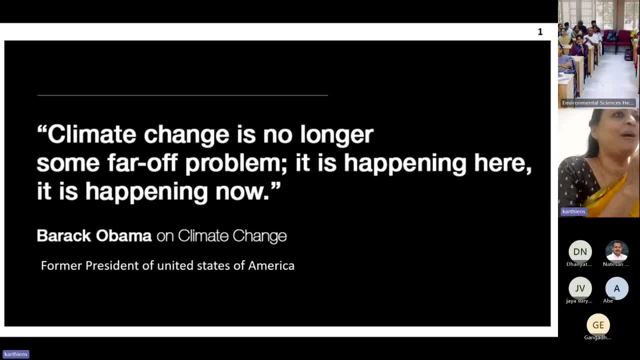 First of all, I thank you, Barani, ma'am and HOD, ma'am, and all other madams, And Madam Kalasili, ma'am has organized a training during 2017.. I had an opportunity to attend microbial mediated nutrient transformations, So I had a very good experience and I am happy to inform that I did my MSCIG program in the Department of Soil Science and Agriculture Chemistry in TNAU. 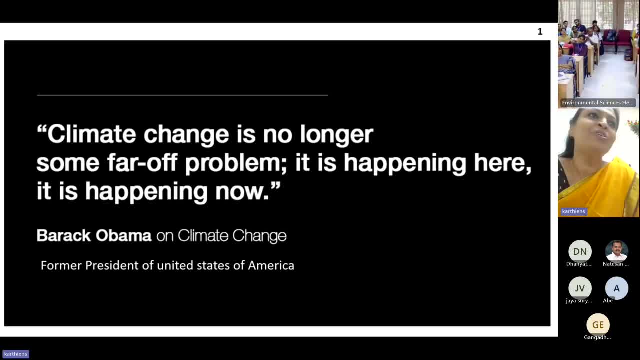 Under Dr Chalmuthu, sir, But unfortunately I was denied a posting in Kerala, in Tamil Nadu Agriculture University, as we don't have a permanent address here And I didn't have an opportunity to work in this university. So I was earning to work in this university, But I was that time when I appeared for the interview, our vice chancellor sir. he asked me. 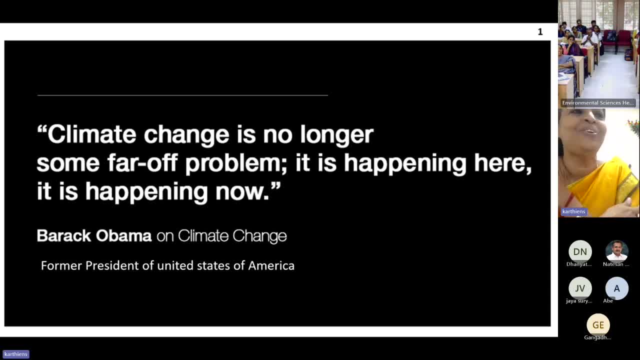 why did you come here, Go to your place, Like that he told. Then I went, But I offered- And I've been here for more than 30 years now And I even have contact with because you really- to be a member of our alumni or to be a student of Tamil Nadu Agriculture University is really great. 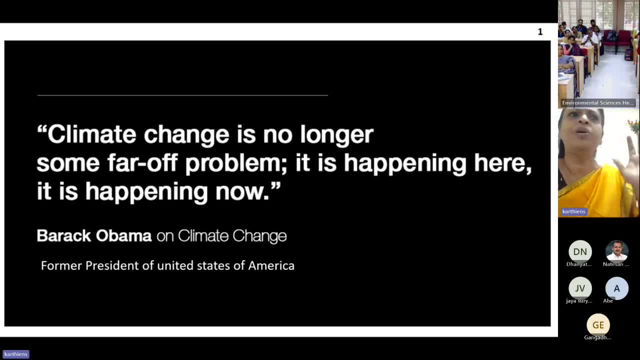 And the basics. what we learn from here will be useful to us in all our endeavors. And when you come to our university you can see the difference. You have all the facilities here. We don't have that much of facilities and even the funding and everything is very difficult. 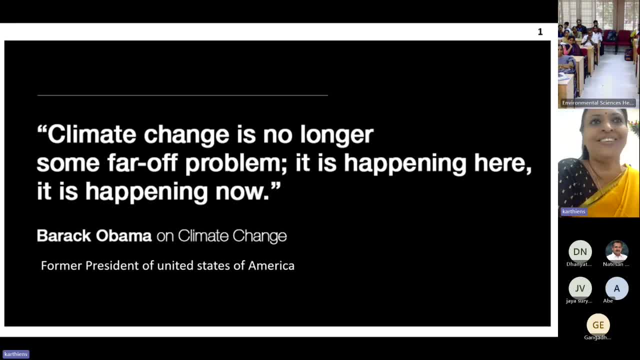 So really, we should be very proud To work here, To work here, work in this great university. okay, so this. i'm also very happy to deliver a lecture on the climate change. as the time is very limited, i'll rush up through the some of the slides, though i. 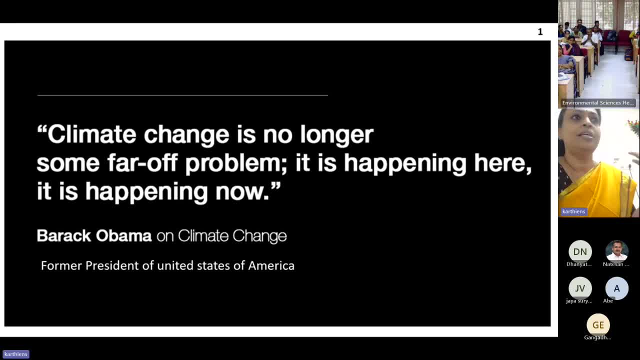 am not a climate scientist. i, uh, i thought, instead of talking about organic menus and all i can talk about climate, carbon sequestration, as this is the environment department of environmental sciences. so we know that we are facing the problem of carbon accumulation, that is, accumulation of 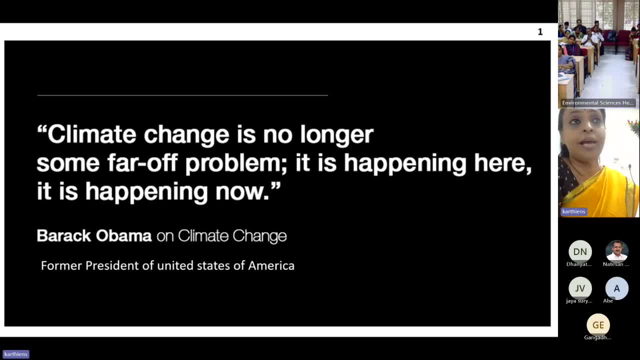 carbon dioxide and emission of carbon dioxide and greenhouse gas emissions, and so many debates are going on and we know that climate change is no longer some far-off problem. so it is happening now. now it is happening and it is the time that we have to intervene and all our cultural operations. 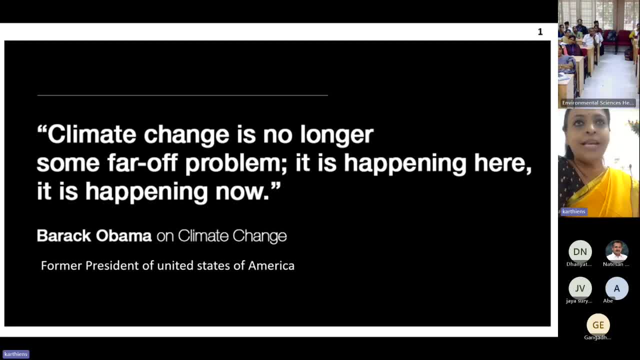 agriculture operations should be focused on a climate resilient agriculture. we have to manage all the activities, or activities in order to cut short the release of carbon dioxide into the atmosphere and also to seek the carbon dioxide that is present in the atmosphere. so for that we have to work. so the 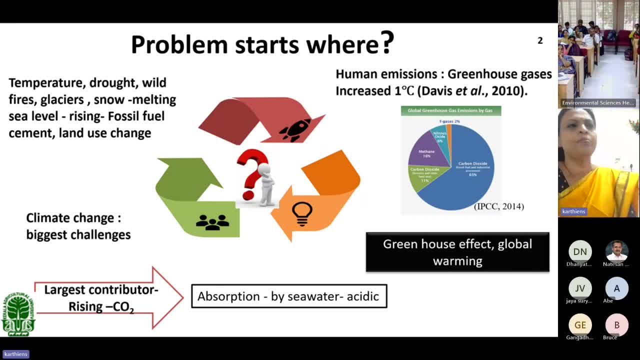 problem starts where. so we have the. we have seen so many problems. so, as mentioned in the papers and in the media, we are seeing that, because of the increase in the carbon dioxide level, there is an, there will be a future increase in the temperature, glacial melting, complete drowning and all these. 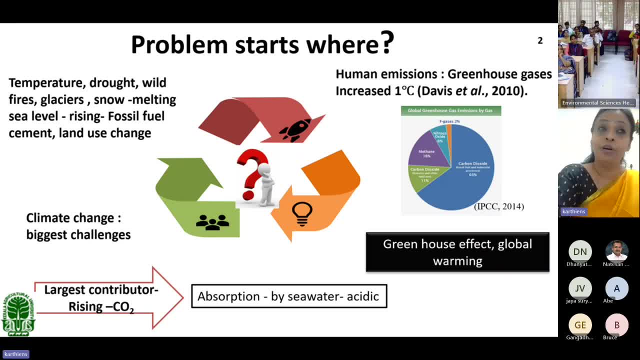 things: what we are threats, what we are going to feel of, uh, in future, what we are going to face- all these things. so it is one of the biggest challenge in the days to come. so we have to manage it. one of the thing is: how can we manage? we are as agricultural scientists. we have to control certain 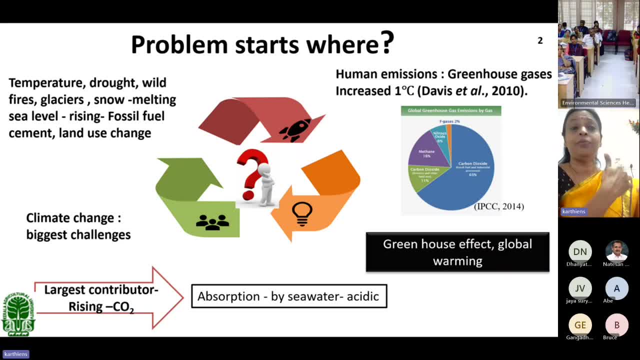 operations and we have to improve certain. we have to manage such that the carbon fraction, that is, the carbon dioxide, has to be fixed into the soil so that we can reduce the level of carbon dioxide in the atmosphere. so that is the need of the day and we have to focus all our attention for the 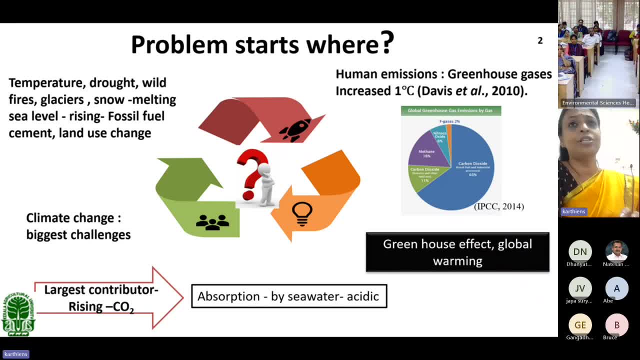 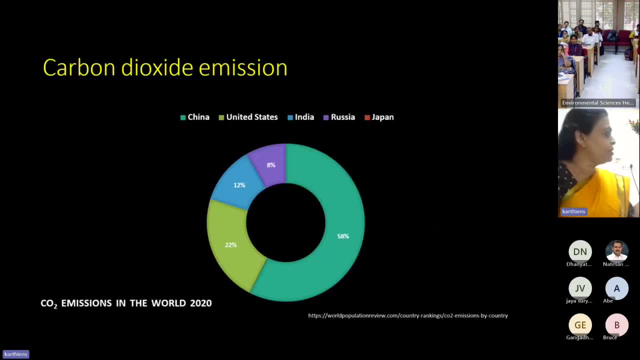 sequestration. that is why i have chosen the topic: carbon sequestration for a climate resilient agriculture. so that is the present day need and we know that our countries are emitting so much of carbon dioxide. we have been talking about carbon trading, carbon credit and so many agreements and 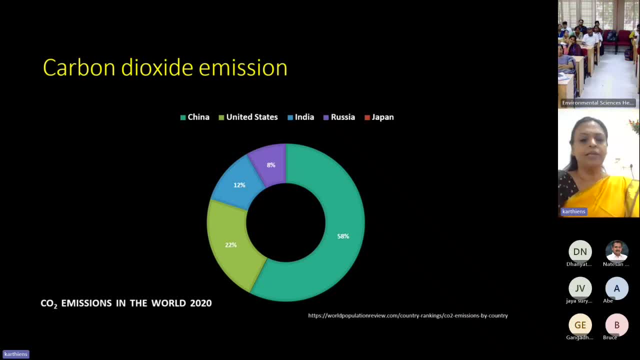 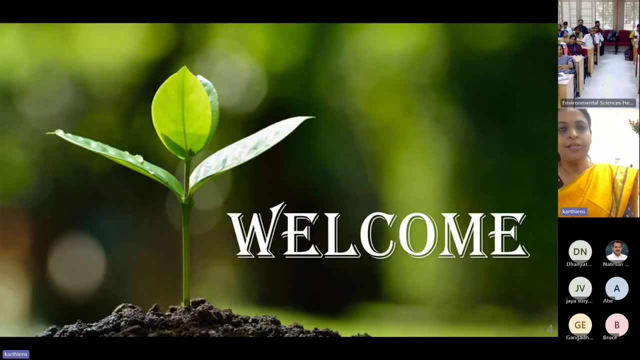 all which we can go through it and we can see that uh majority in the case of china, that is the country that is emitting carbon dioxide and with this, with this introduction, i will- i would like to welcome you all to the topic: carbon sequestration for a climate resilient. 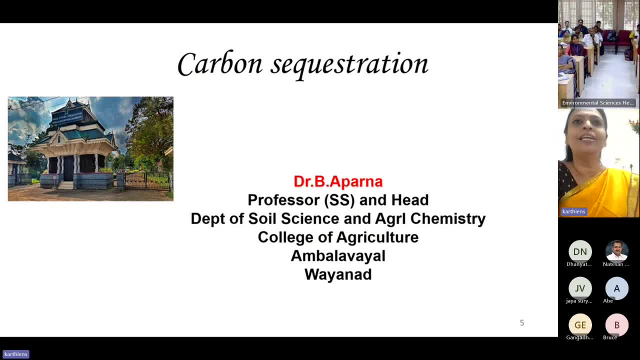 agriculture, as um madam has told that recently i've been transferred to college of agriculture for accreditation purpose. i'll be shortly going to my own department again for a short period. i am now in vayana and you can. i am inviting you all to vayana. it is a nature's gift you should see. 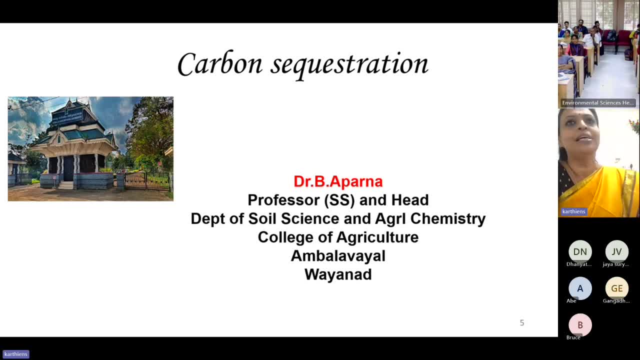 vayana. it is a very beautiful place, and we had also organized a international flower first properly, which is amazing. your office is so beautiful and you can see the hoffeley ground is now open also, so at any time you can come and visit us then. so these are the some of the activities that that. 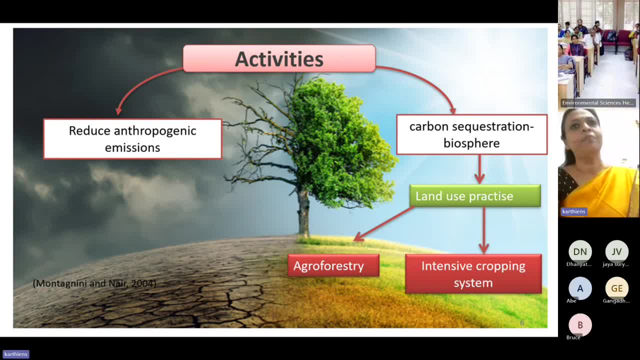 has resulted in the uh accumulation of the carbon dioxide. so from our ug program we've been studying. so application of the pesticides, fungicides, fertilizers did not, judicious application of the fertilizers and also those frequent tilling of the land, all these will increase the carbon content. 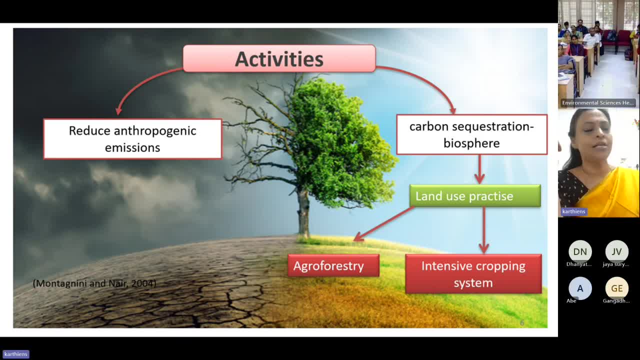 in ICR has recommended the zero budget. natural farming, natural farming, natural farming, so many farming systems in order to give minimum disturbance to the soil and to preserve the carbon that is present in the soil. That is one of the important aspect. So also what happens? we are burning the agriculture residues. 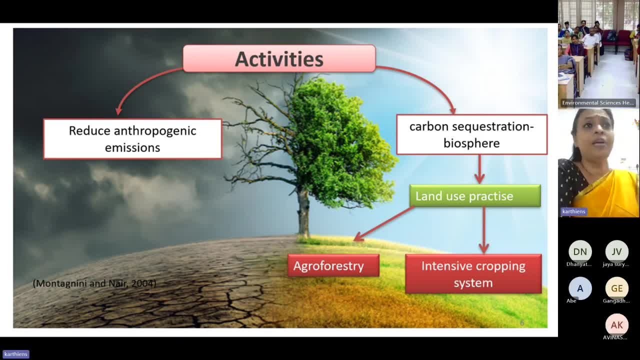 So what the farmers? they do. So we have to create awareness to the farmers that we have to prevent their action of burning the agriculture residues, which again adds to the carbon dioxide in the atmosphere. So what we are focusing is carbon neutral agriculture. So you might have seen. 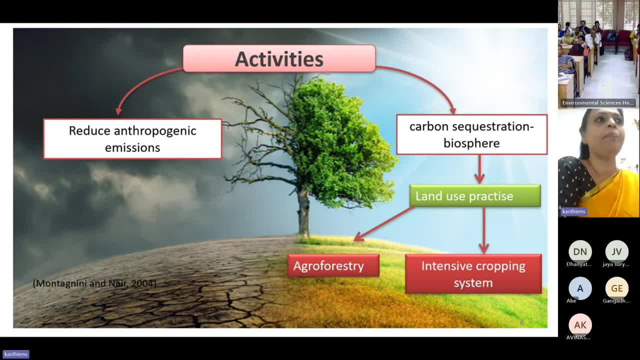 So neutralizing carbon is not an easy task and it won't take it to happen within one or two days. It takes a lot of time. carbon neutral agriculture. So now it is said that net carbon, net zero carbon agriculture, That means you have to bring the carbon level in the atmosphere to a neutral level. 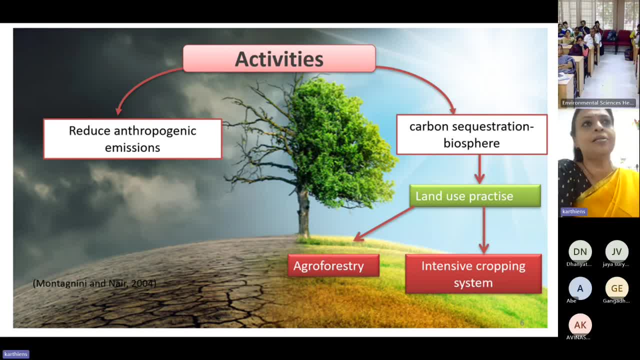 So that is called neutral, That is carbon neutral agriculture, and we have to promote all the activities in order to fix the carbon and make it to your neutral level. So in the, so in Kerala, so we have so many plantations and so many. 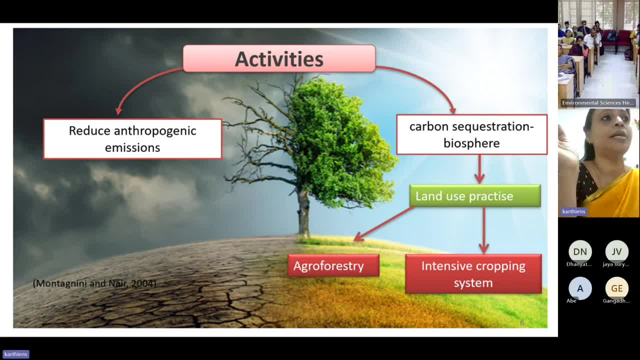 So we have the coconut plantation, So that is present in all the states, like Tamil Nadu, Karnataka, Andhra Pradesh and all. So, with a special reference to coconut, I'm going to highlight this presentation. So now we can. So what are the sources of carbon dioxide emissions? 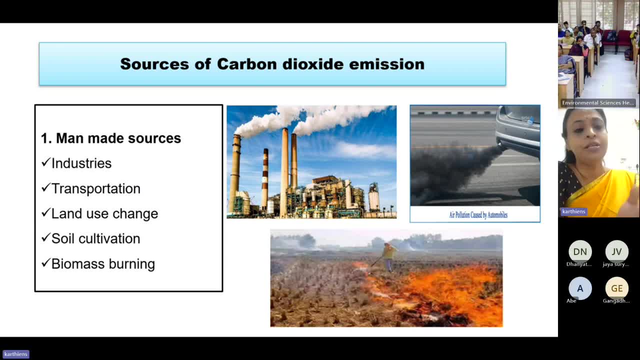 We have the manmade sources, like industries, transportation, then land use change: soil conservation, soil cultivation, That is an important thing. Tillage is very important thing and biomass burning- That is also another important mistake. What we are doing to improve the, to contribute the carbon in the atmosphere, the natural, 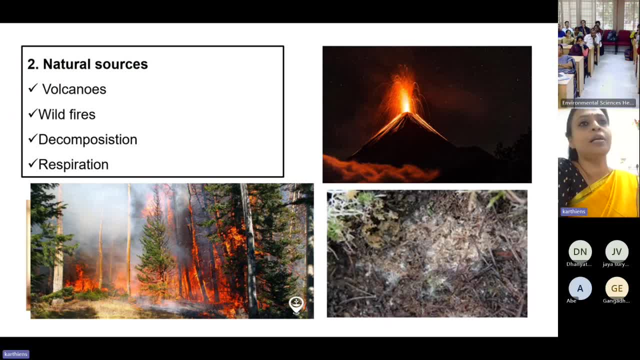 sources also. naturally there will be the addition of carbon dioxide in the atmosphere. So by the process of volcanoes, wildfires, decomposition, decomposition of carbon dioxide, we can reduce the carbon dioxide. So we have the process of decomposition. We need that. 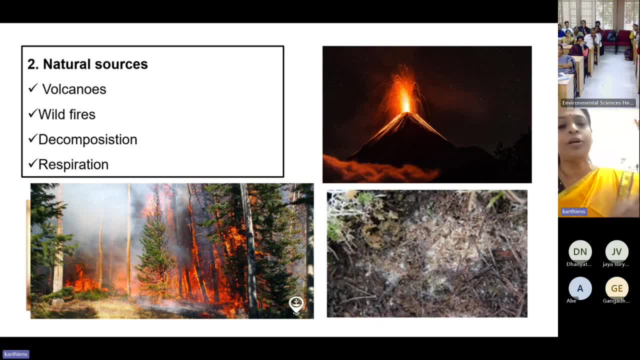 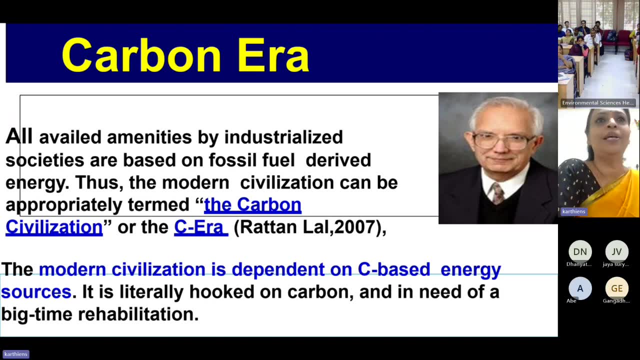 We know that when it is decomposed, carbon dioxide is the final product that is evolved, that goes into that atmosphere and also respiration. So now at this, we should call this as an carbon era, because our great scientist, Dr Athanlal, he has focused on the carbon civilization and also the carbon era. 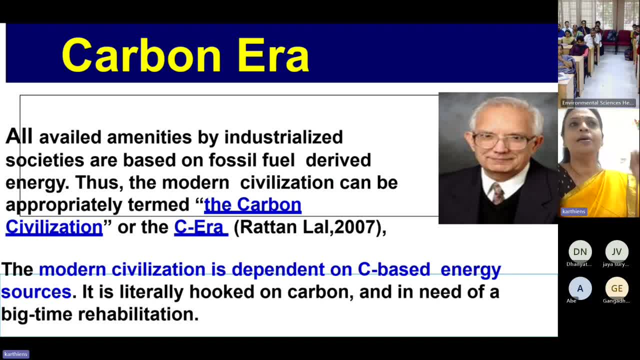 He has also highlighted. so many of the works have been focused on the carbon sequestration. He was one of the scientists who- Who was one of the scientists who has highlighted- emphasized the need for sequestering carbon and also to reduce the level of carbon in the atmosphere. 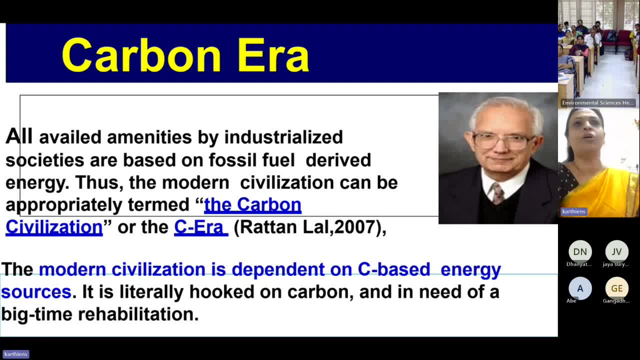 So he has mentioned that this civilization is called as carbon civilization or it is also called as carbon era. You know the achievements of Dr Ethan Lark and he said that our economy, modern civilization, everything is dependent on carbon-based energy sources. So this is another important thing, what we have to think about it. 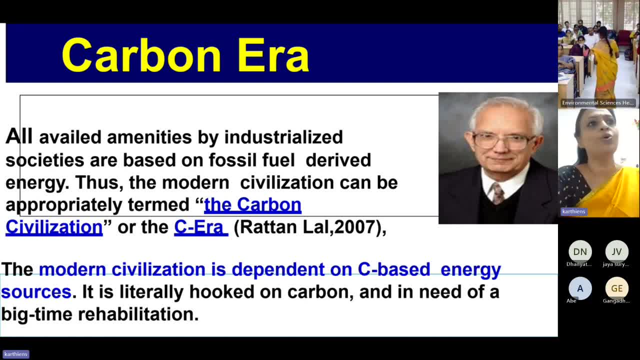 And sir has. we know that there are so many fractions in the soil. So we have the organic carbon, water-soluble carbon, residual carbon, so many fractions of carbon. So normally, as a student of agriculture, we'll be thinking about organic carbon status. 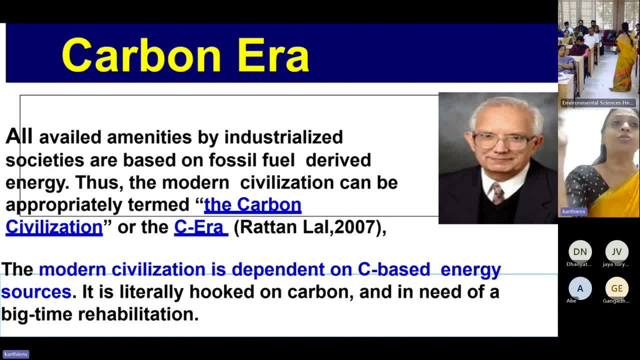 Whatever management practice, we will try to improve the organic carbon, But there are so many fractions of carbon and so many fractions of carbon, So this is another important thing, what we have to think about. So the biochar- Shahida was mentioning about biochar. 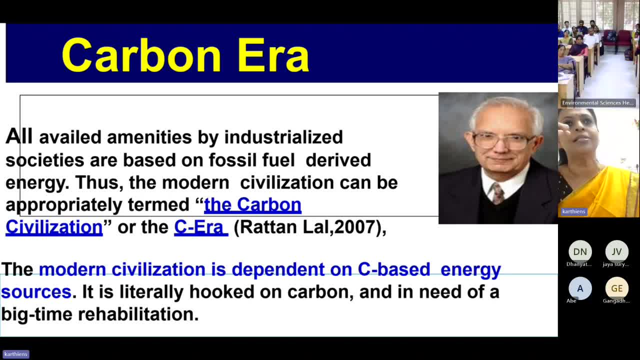 So the carbon that is present in the biochar is the recalcitrant carbon that is available throughout. That is not amenable for decomposition. So there are so many fractions of carbon are available. So our ultimate aim is to improve the carbon fractions of the soil. 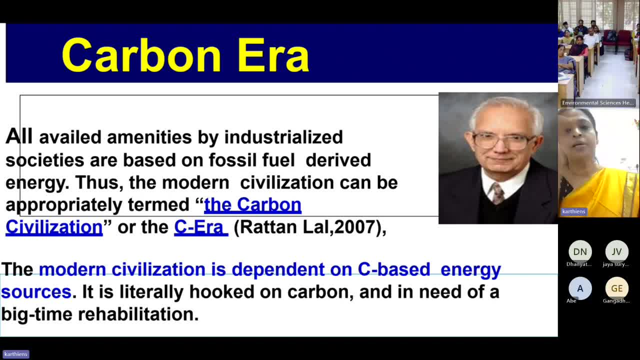 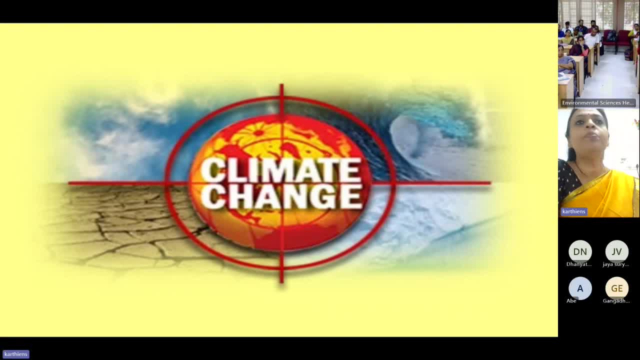 So many fractions are available. So those are all highlighted by Dr Ethan Lark. And so climate change. So another problem. What is the problem of this carbon accumulation in the atmosphere? So one is the climate change. We know that the last year, January, you might have received rains. 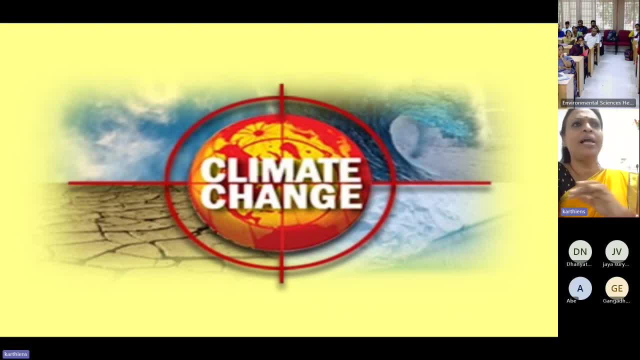 This year you won't get rains, So it is not uniform. So and erratic Monsoons are highly erratic, So our agriculture is dependent upon this erratic climatic change also, So we cannot predict what is going to happen next month and what will be the. 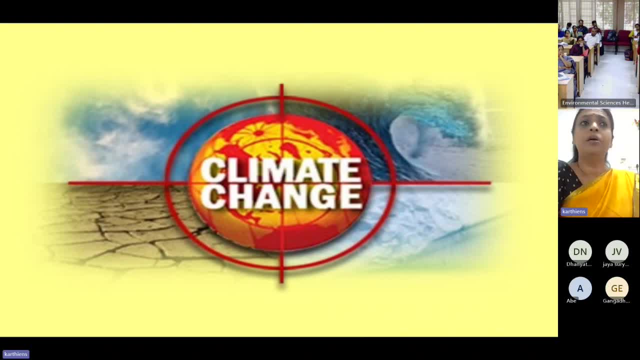 So during daytime we experience very high temperature, With Which earlier days we didn't experience so much. These are some of the impact of climate change- carbon accumulation in greenhouse gases. So the climate is ultimately changing and you don't get a uniform pattern of climate over a season. 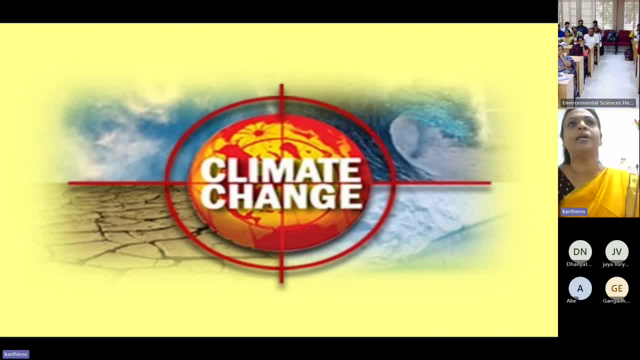 And the meteorologists are facing so many problems that they cannot predict the climate change and recommend to the farmers. So that is it. We will say that there will not be rain, but there will be rain during May or April. So that is so. monsoons. 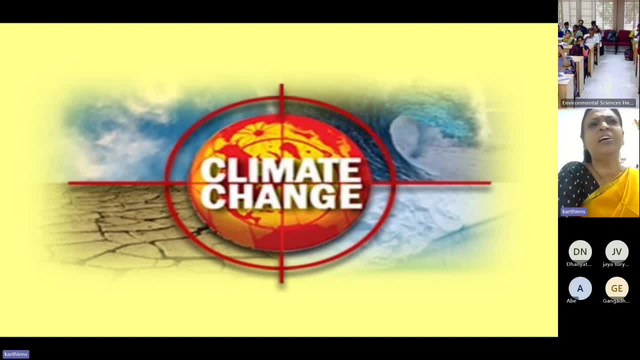 So you take in the case of Kerala, During 2018 and 2019, consecutively, we received floods, So floods means complete devastation and all the agricultural lands and everything were underwater. So what happened is all the soil properties and everything, loss of nutrients. all these things were reported. 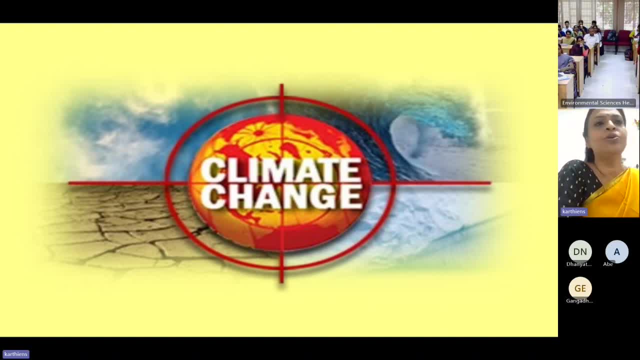 So that was one typical example for the climate change. So now we have formulated a project- the potential impact of climate change on flood. Like that we have formulated a project. We have taken the soils, we have analyzed and we are predicting what can be. 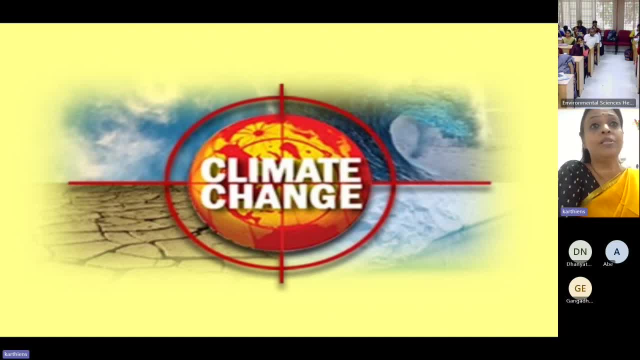 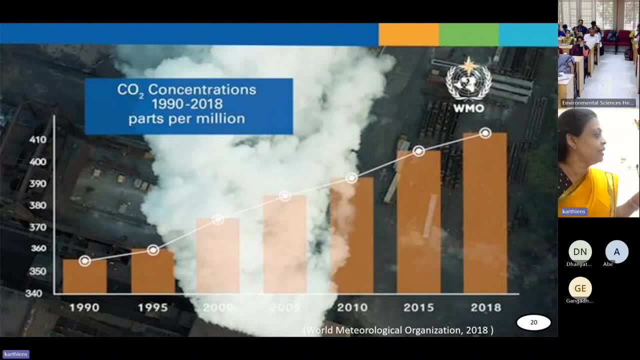 Like that, in which we can find out that carbon is very important, which has contributed to the changes in the climate. So this is another important thing. So we can see that from this figure, we can see that there is an accumulation of the carbon over years, from 1990.. 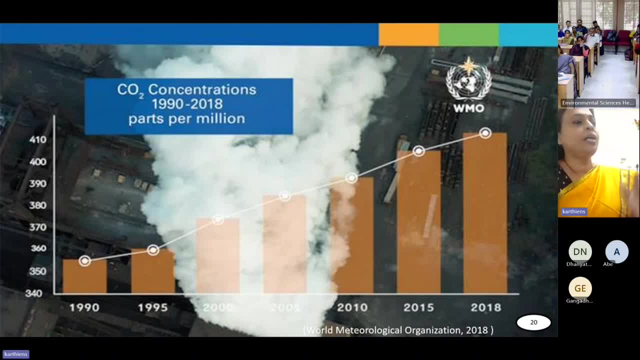 So this is a data that is from World Meteorological Organization, WMO, So this department. So we can see that the carbon dioxide accumulation, the content PPM, So we can see that the carbon dioxide accumulation, the content PPM. 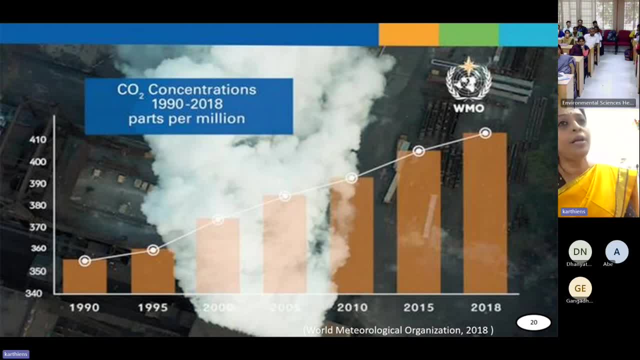 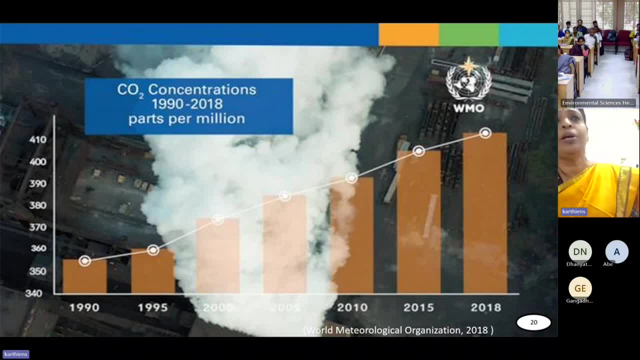 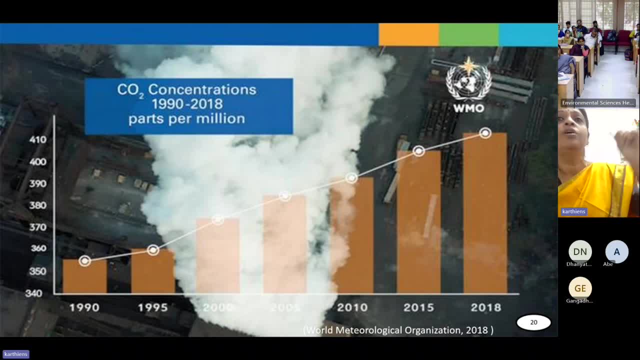 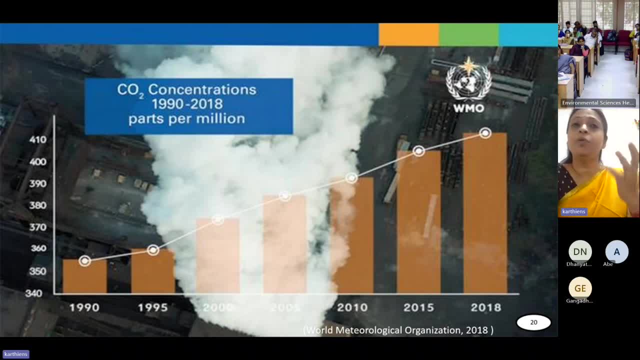 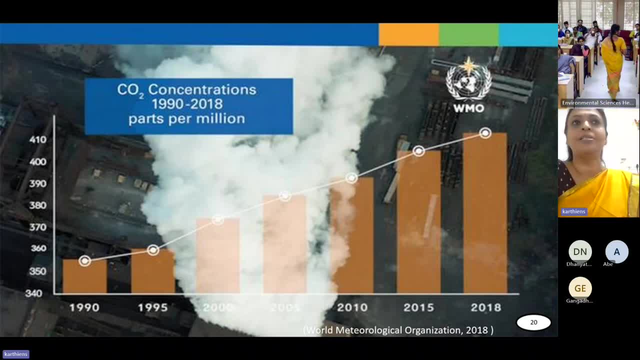 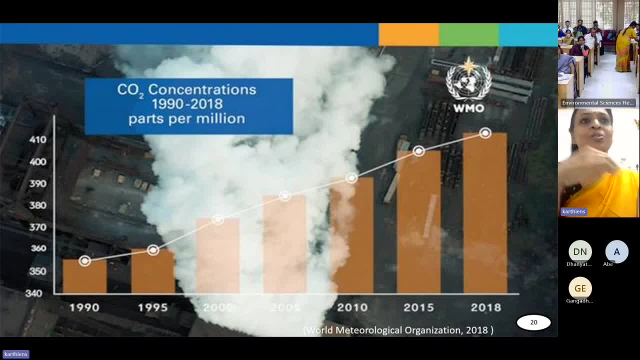 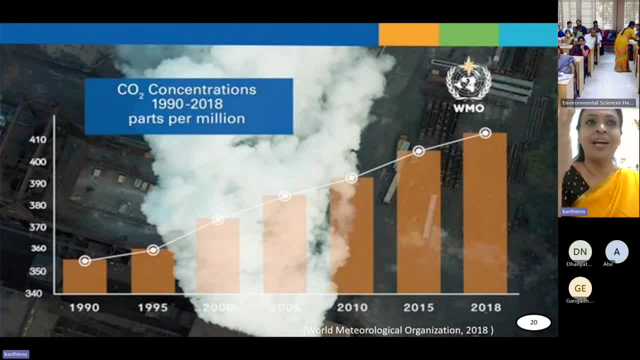 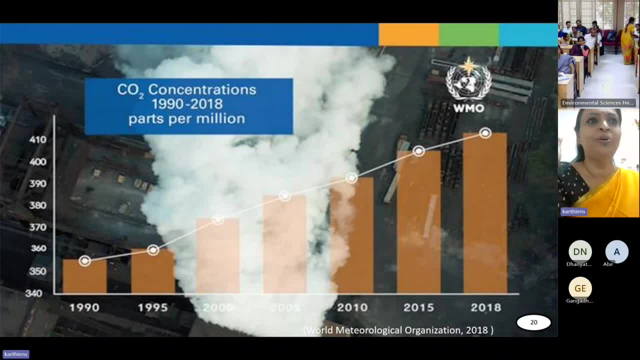 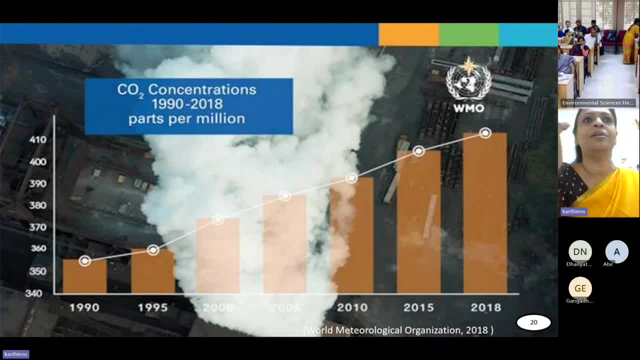 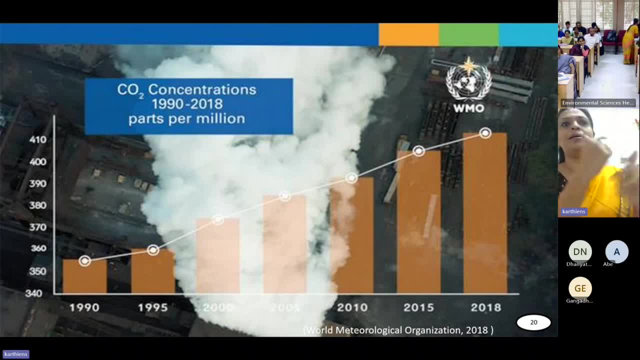 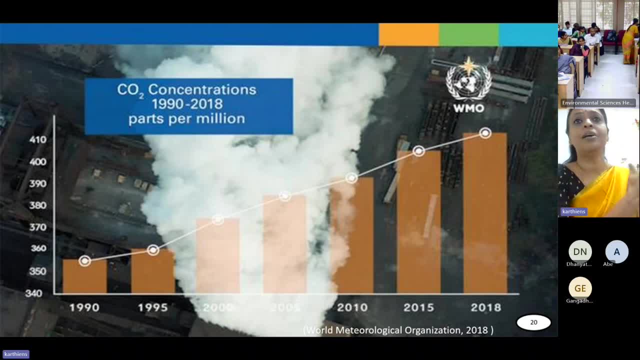 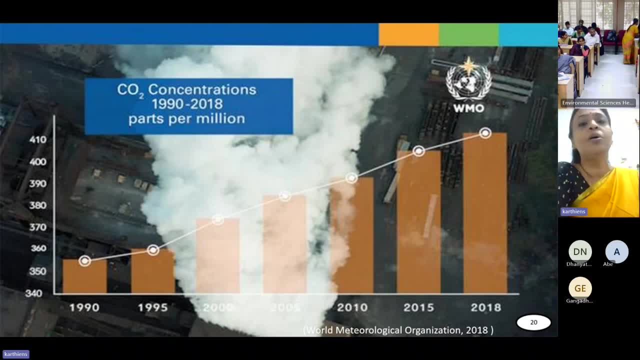 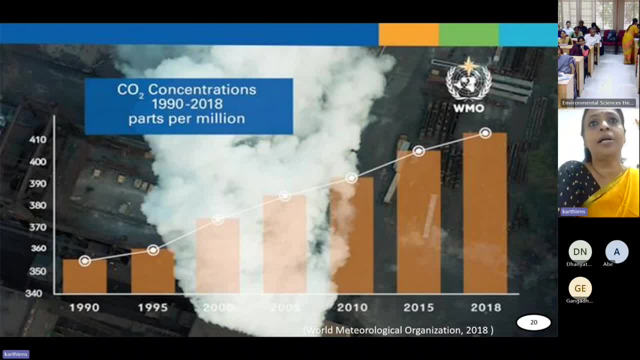 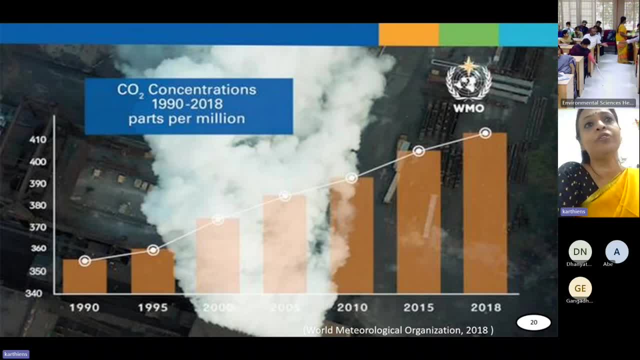 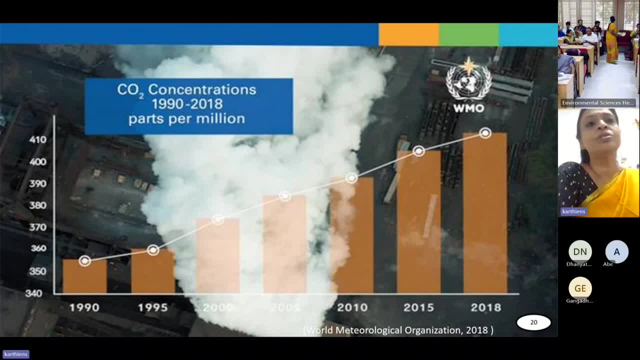 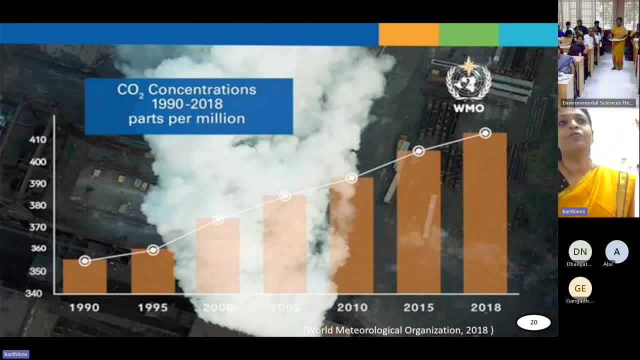 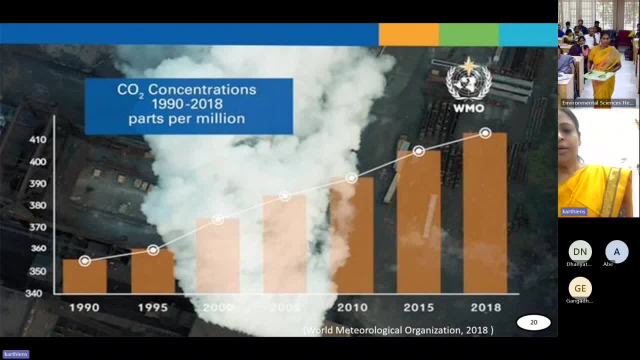 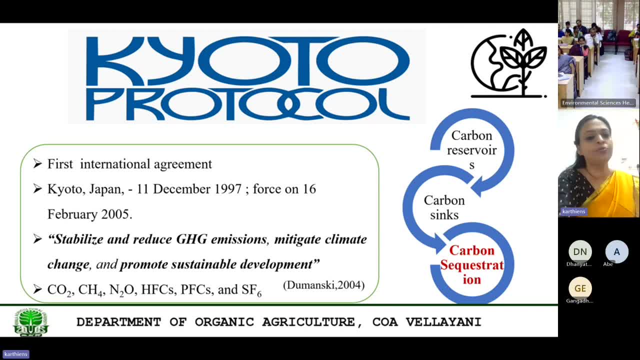 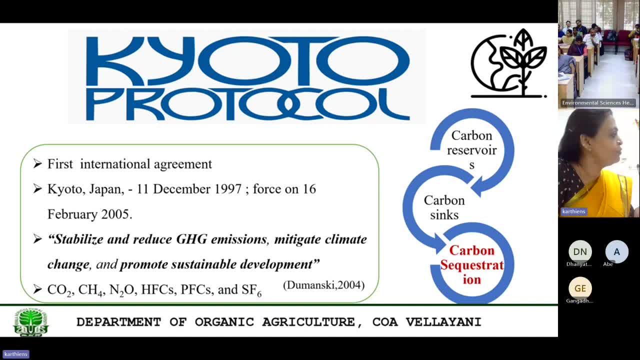 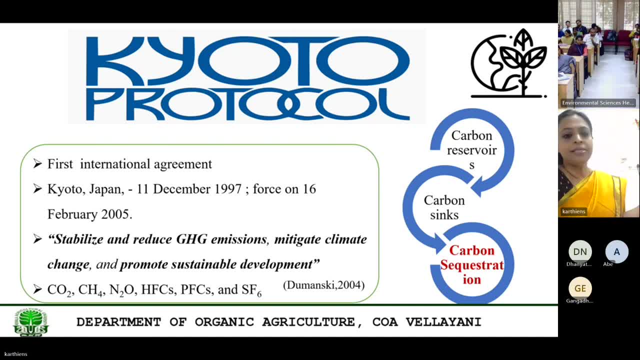 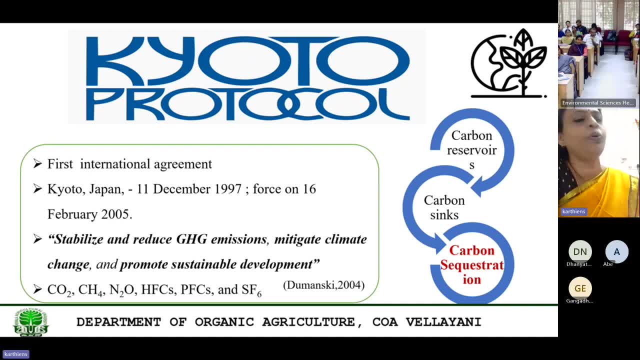 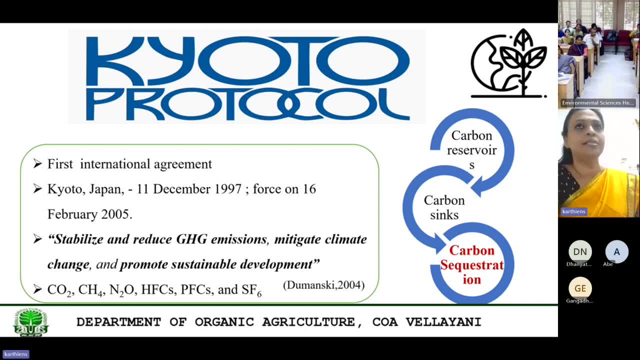 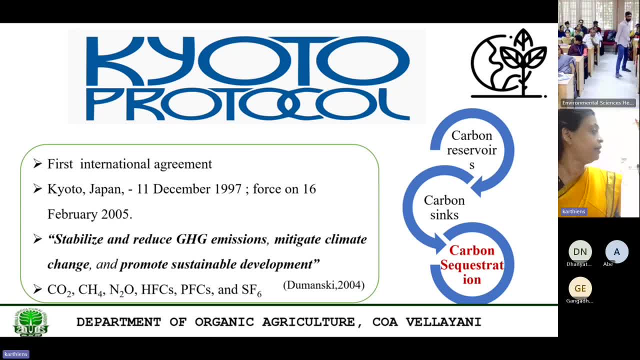 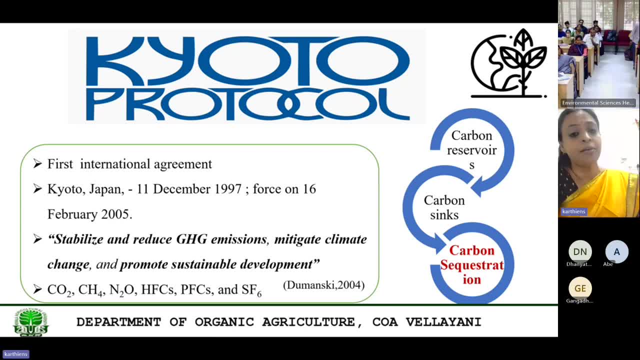 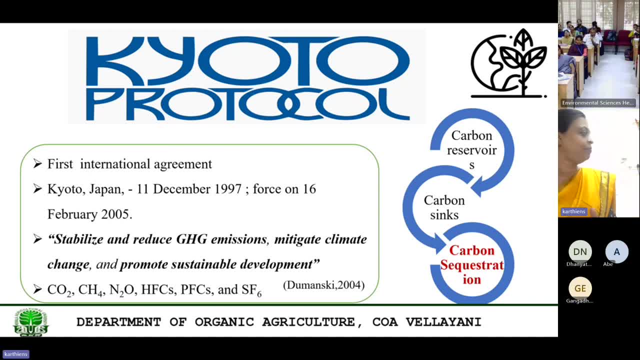 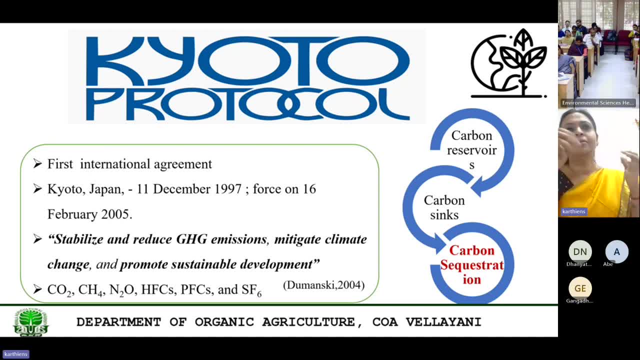 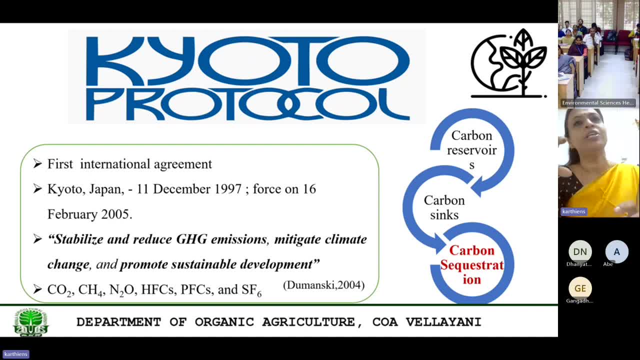 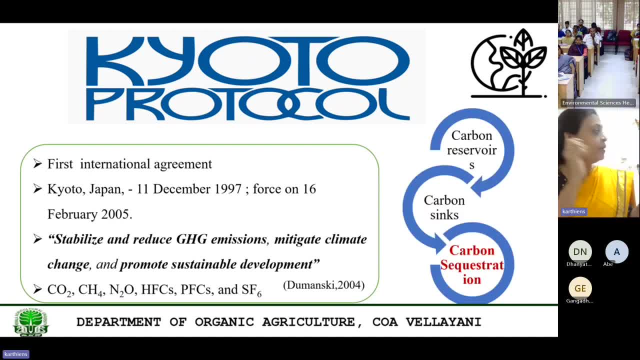 as well as to reduce the carbon emission. so carbon reservoirs: we have to identify the carbon reservoirs, carbon sinks and also carbon sequestration. so the ultimate aim: it is given in red that we have to sequester the carbon. what is carbon sequestration? fixing of the 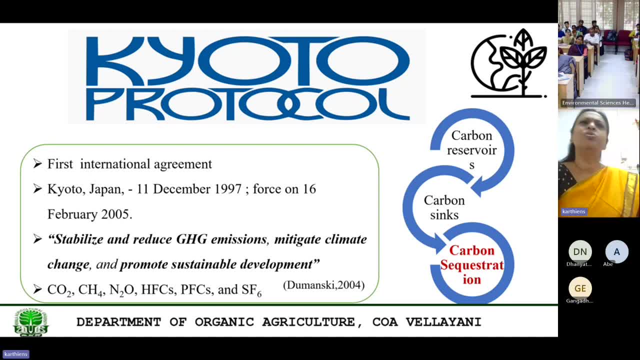 atmospheric carbon in the soil. that is called as carbon sequestration. so by simple method, by growing plants, by growing as told the bamboos or plantations, and all we can fix the carbon, add to the biomass, to the soil, and thereby we can improve the practice of the carbon. so this 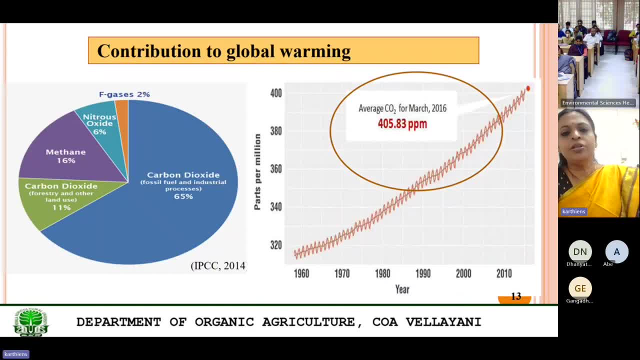 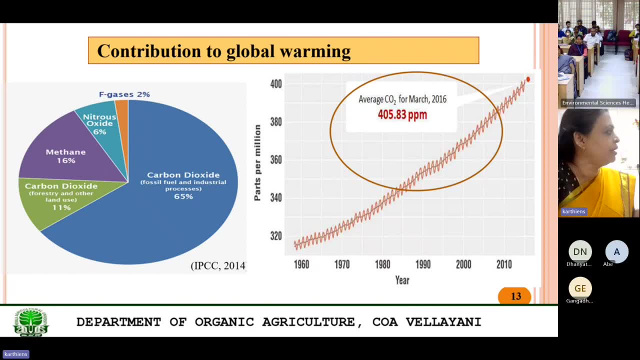 is one of the simple method, and so these are the factors that contributes to the global warming. also, you can see that. what are the gases? carbon dioxide, carbon monoxide, the nitrous oxide. all these gases will contribute to the global warming. global warming is the is the word that is used by. 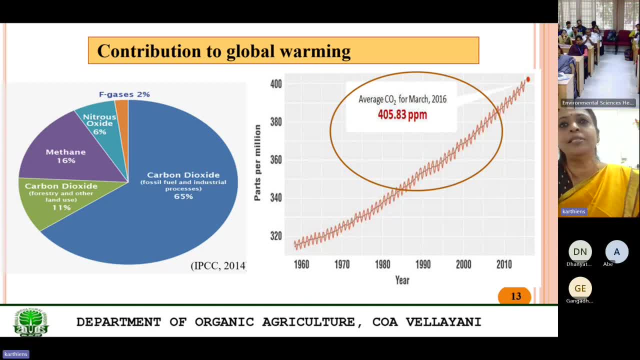 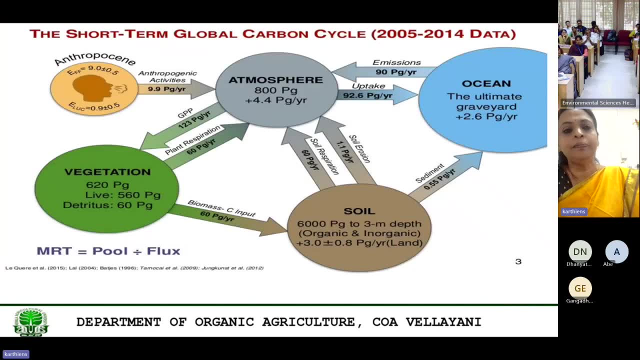 various media to threaten. of course it is a threat to all the humanity, so it has to be taken into global warming so we can improve the practice of the carbon. so this is one of the simple method, serious consideration. we have to give full attention to global warming and work accordingly. 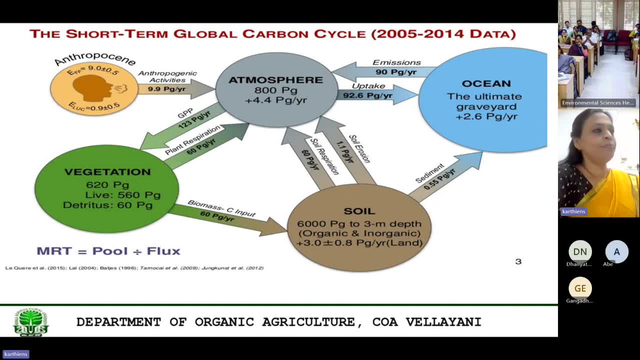 so these are the some of the amount of carbon dioxide, that is, peter gram of carbon that is released. you can see that vegetation, soil, then ocean, atmosphere and all these things. so the global carbon cycle. so these are the carbon cycle that is operating between the atmosphere, soil. 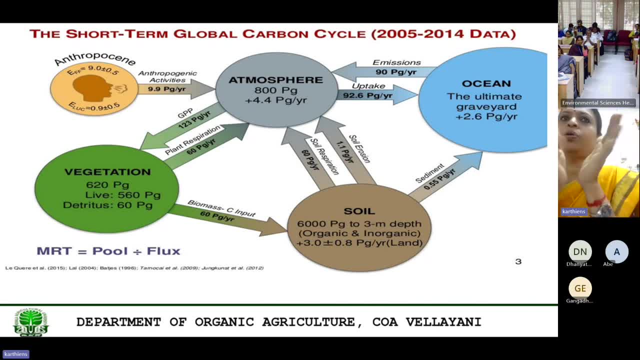 terrestrial, oceanic and out. so sequestration is also not only terrestrial sequestration. we have the marine sequestration, so many other types of sequestration, so sequestration can be done either by the plants or by the water bodies, or by any thing, in order to reduce the carbon content in. 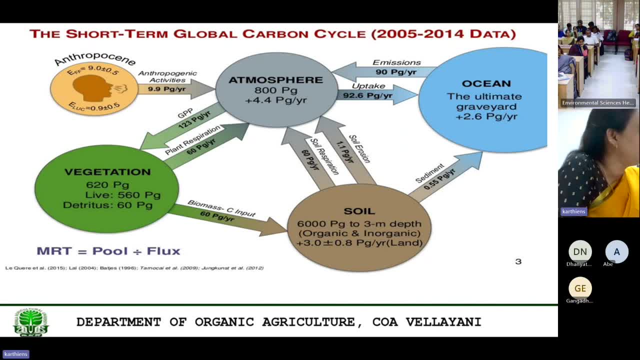 the atmosphere. so these are the. you can see the balance between the emission as well as the uptake, as still there is an imbalance that exits because of the uptake is less and the emission is more. so that is why we have to focus our attention on the sequestering of the carbon. so this is the 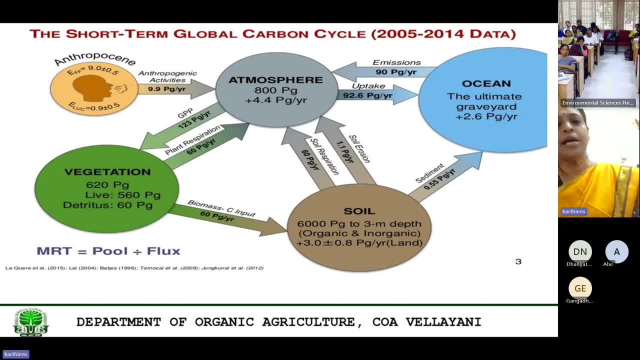 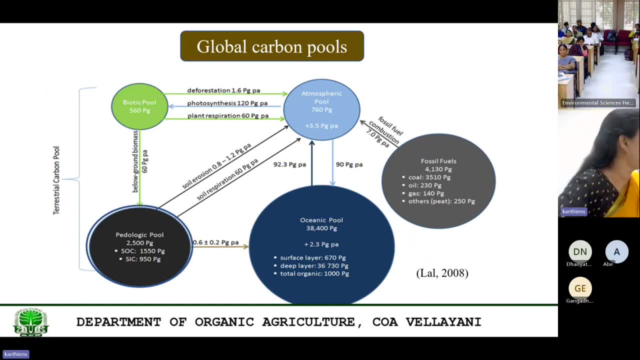 this is one of the important global carbon cycle data. then these are the modified form of the global carbon cycle. so we have the biotic pool, abiotic pool, then oceanic pool and pedologic pool. all these things are fossil fuels. so this is the data statistics. this ppt, i can give a give it to some one of you can. 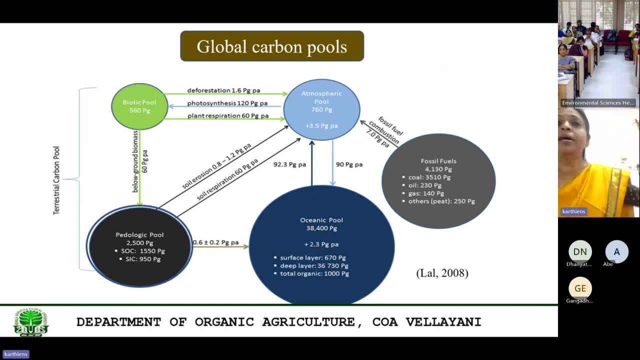 have the statistics also. this was also. this was given by rathan lazar in one of the presentations. uh, in the year 2008, what was the amount of carbon that is released in the atmosphere? so this is the amount of carbon that is released in the atmosphere. so this is the amount of carbon that is released. 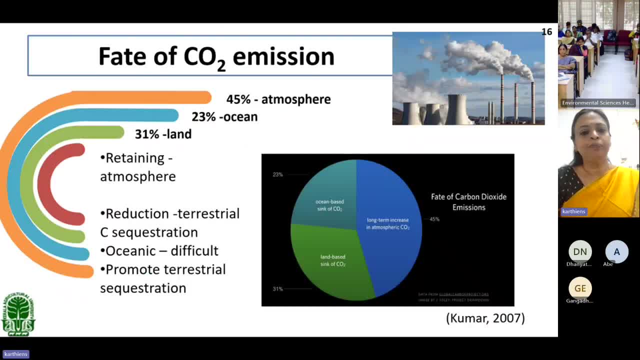 by the various um pools. then fate of carbon emission. so we we can see the uh: 45 percent is atmosphere, 23 percent is the ocean, that one is the land. and what is the face of a fate of a carbon? so that, uh, that in that impacts on the climate change and erratic uh climatic um modifications as well as. 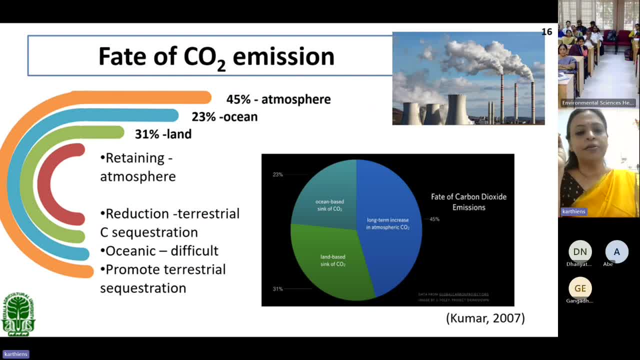 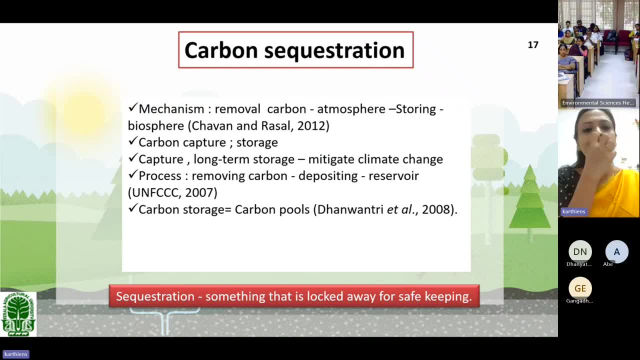 heavy floods- all these are some of the ill effects of this carbon dioxide emission. so now we come to the topic that is, carbon sequestration. so carbon sequestration is the removal of the atmospheric carbon and storing in the biosphere. that is called as carbon sequestration, and it is 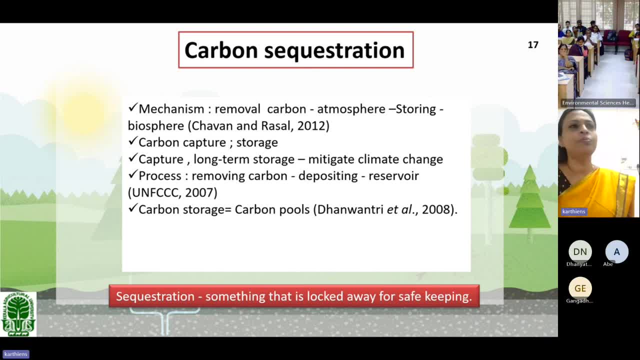 also capturing of the carbon and storing in the soil. so there we have so many uh terms. also carbon stock and the carbon pool and different related terms are there. so you know the difference between biomass and necromass. as madam is here, i should not ask: what is biomass, what is necromass? so biomass. 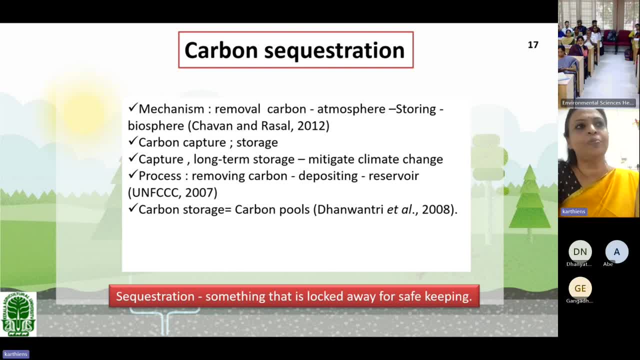 the living organisms. so carbon that is released by the through respiration and decomposition, that is called as biomass, necromass from the dead, organic, the dead biomass, that is called as necromass. so that also contributes to the carbon dioxide to the atmospheric level. so that is also another. 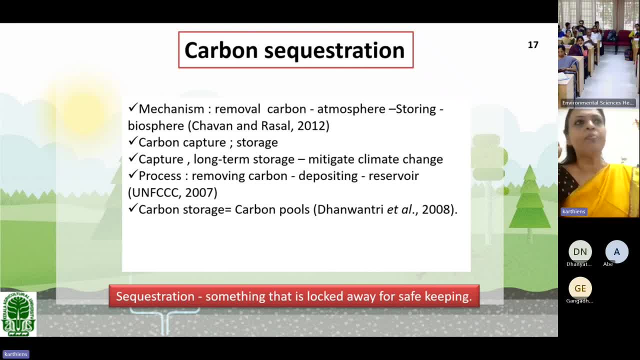 human being. so when we die, we also decompose and carve a certain amount of carbon dioxide disabled. so likewise the microorganisms, even though they are, if they are alive, they will decompose all these organisms. carbon dioxide is released and also the necromass. when the microorganisms itself will die, that will also release the carbon. 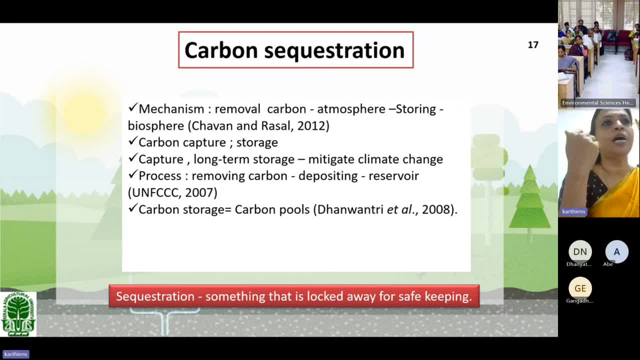 dioxide. so we might have estimated your respiration, carbon dioxide, respiration activity, fumigation technique and all by by, by killing the microorganisms and then estimating the carbon dioxide emitted. then carbon storage, that is, carbon is stored in, that's different carbon pools. so we have so many carbon pools are there in the soil, as well as the oceanic pool, terrestrial pool and out. 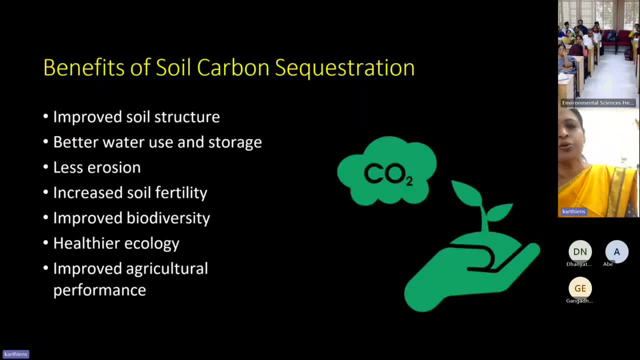 also as different fractions, also the carbon. so the carbon is being stored, stored. so benefits of the soil: carbon sequestration. what are the various benefits we have? the improved soil structure, because carbon is the backbone that will improve the soil structure. better water usage and storage. less erosion: when the soil structure is improved, there will be less erosion. increased soil fertility. 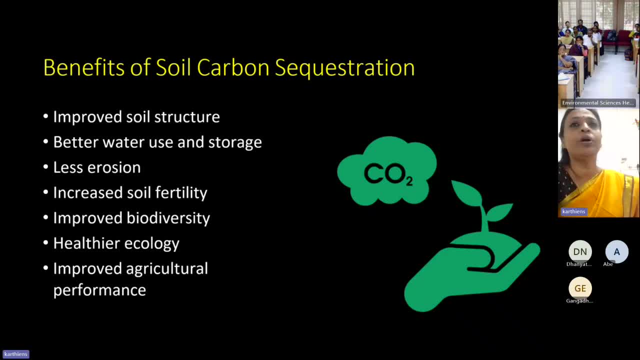 carbon is the backbone and you can assess the quality of the soil with the carbon content. if the carbon content is more, then you automatically you can say that the soil is highly fertile. then improve the biodiversity. of course, carbon is related to the biodiversity. if there is more carbon, more microbial dynamics will be there and healthier ecology and improved 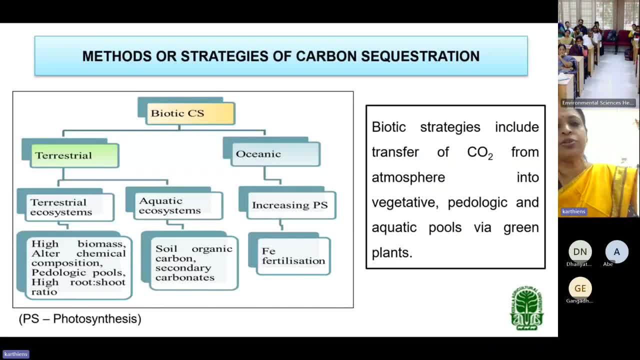 agricultural performance. so these are the some of the benefits of carbon sequestration and methods of carbon sequestration. we have the various methods like terrestrial and oceanic, biotic method and abiotic. in the case of biotic, we have the terrestrial and oceanic. terrestrial 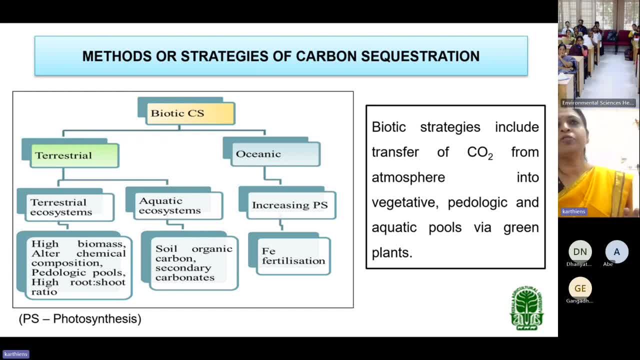 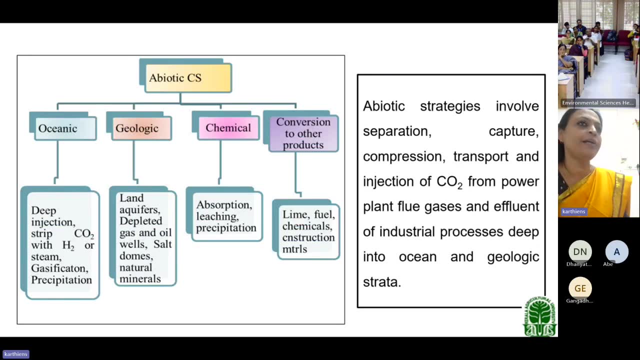 aquatic and all these things we can see. these are the some of the methods, how we uh, in which the carbon sequestered either by the terrestrial ecosystem or aquatic ecosystem, by um, by fixing the atmospheric carbon, then abiotic. abiotic means other factors that are not um with life. they are 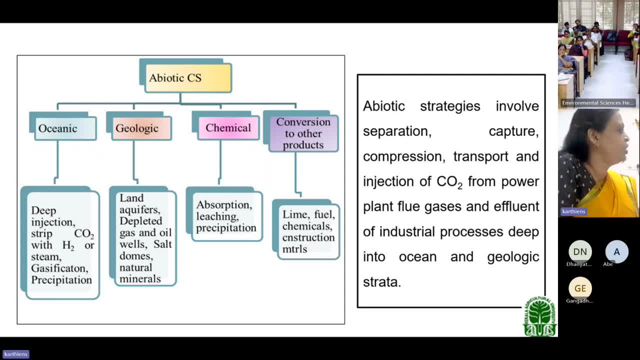 called as abiotic carbon sequestration. we have the oceanic, geologic, chemical and conversion to other products. so oceanic carbon sequestration is there, geologic carbon sequestration? is there then chemical action? then so many process. in the case of oceanic, so many process carbon dioxide is injected into. 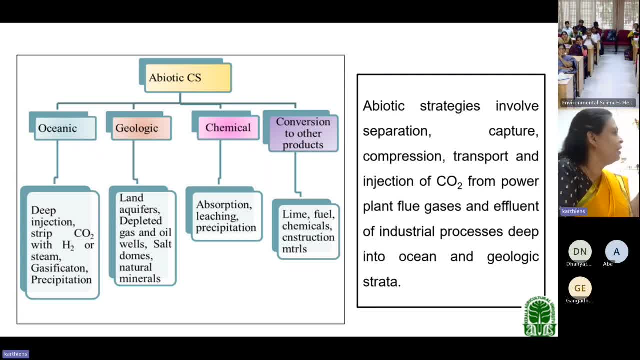 it, gasification, precipitation, all these processes. then we have the geological. in the case of geologic, we have the land aquifers, depleted, gas and oil wells, salt domes and not. then we have the chemical absorption, leaching and precipitation. so that is also another method of carbon sequestration. so 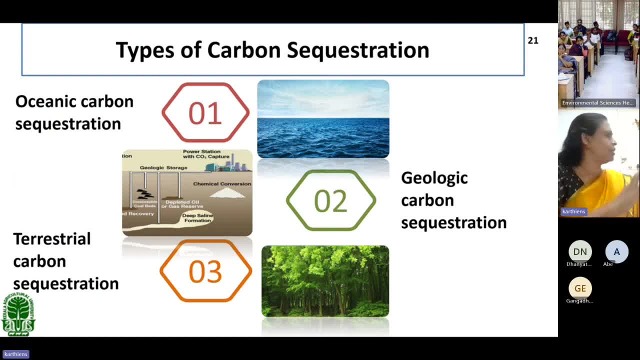 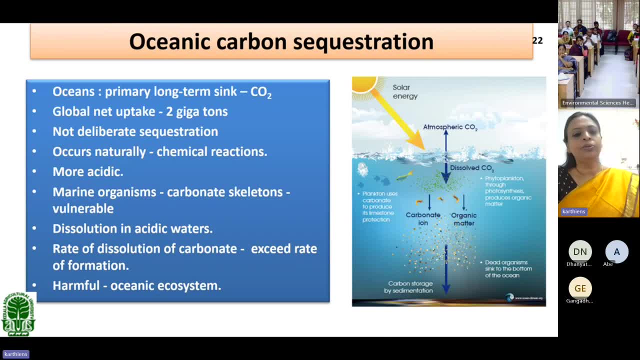 these are the various methods by which the carbon can be sequestered, so this is a clear picture of oceanic carbon sequestration. so this is a clear picture of oceanic carbon sequestration. terrestrial carbon sequestration, geologic carbon sequestration. so by using this, you can see that atmospheric carbon dioxide is. 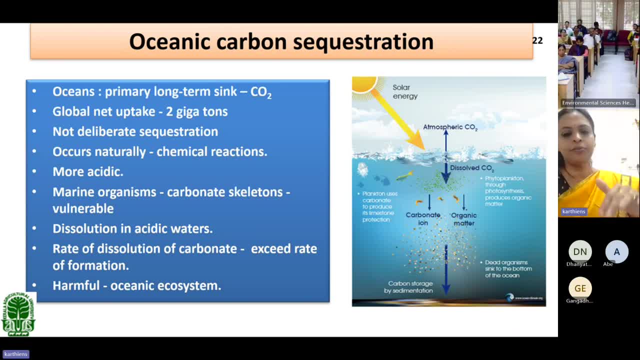 converted to dissolve the carbon dioxide when it enters into this water and then that will be fixed by the sedimentation as well as by the marine organisms. that carbon dioxide will be taken up and that will be also fixed. that is also called. but one thing is, when the carbon dioxide is dissolved, 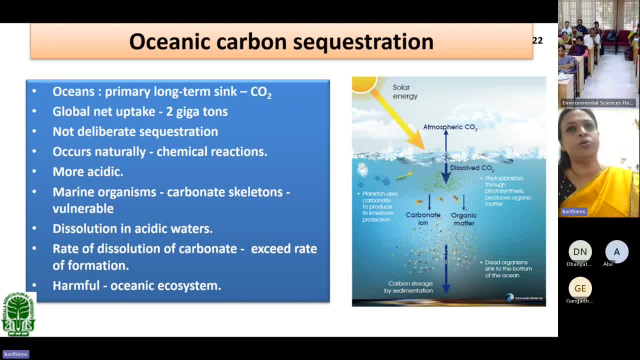 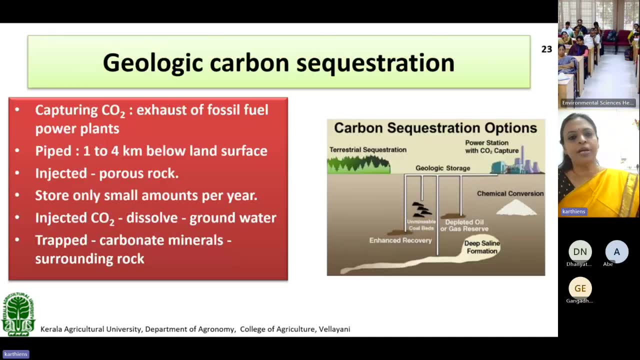 in the water. it produces carbonic acid and it becomes more acidic also. the system will become more acidic, also acidic, so dissolution in acidic waters and that will also causes. so that is also one type of carbon sequestration. then we have the geology carbon sequestration. so, uh, from the figure we 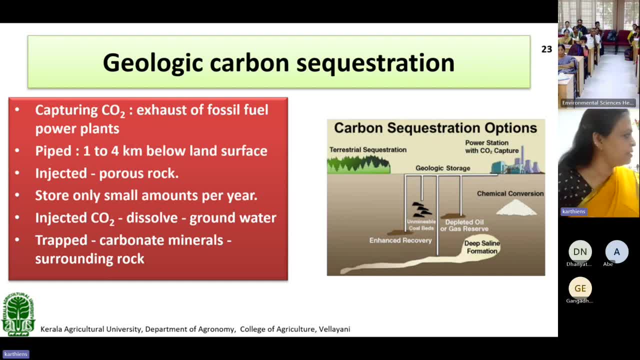 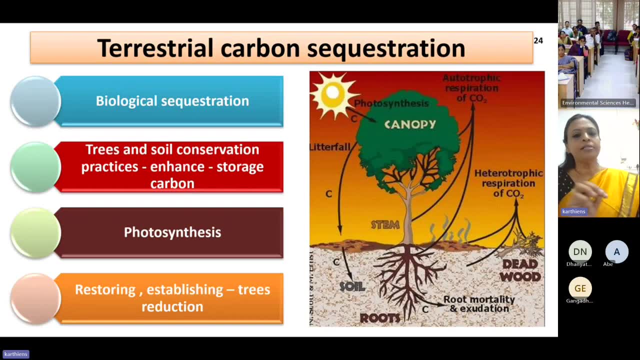 can understand that, um uh, the, in the deep layers the carbon is sequestered and carbon is pumped into the lower layers and the carbon is sequestered and terrestrial carbon sequestration, normally by the biological sequestration by the plants, then trees and soil conservation practices, then 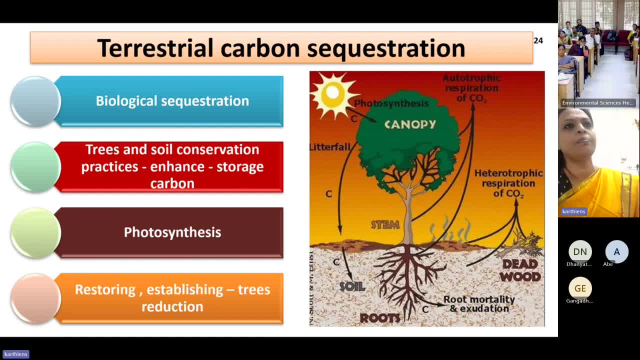 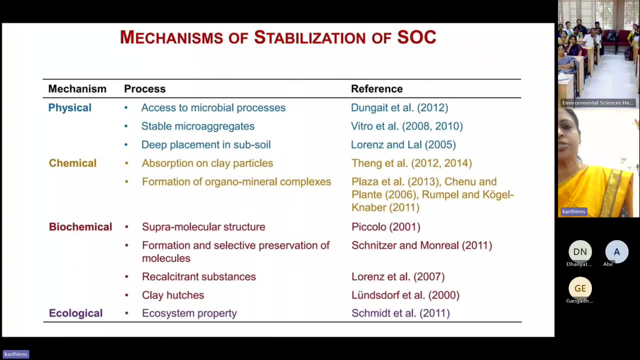 photosynthesis, which is normally a natural process of carbon sequestration photosynthesis. then we have the restoring, establishing the trees. so that is also another method of afforestation programs. all these are some programs which can improve the terrestrial carbon sequestration. so these are the mechanisms of stabilization of carbon. so according to that, we have the physical 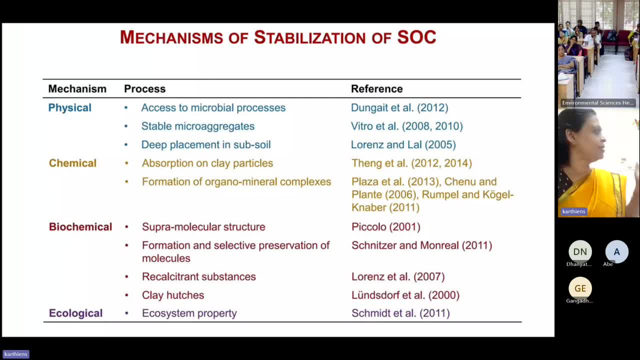 methods: chemical methods, biochemical methods and ecological methods. so these are the various mechanisms, so that should be you by the physical or by the chemical, by by the absorption of the clay particles or organo mineral complexes, or by the biochemical methods, like clay hatches, or by the super. 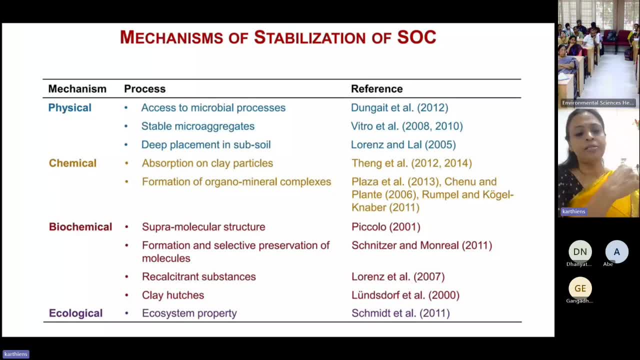 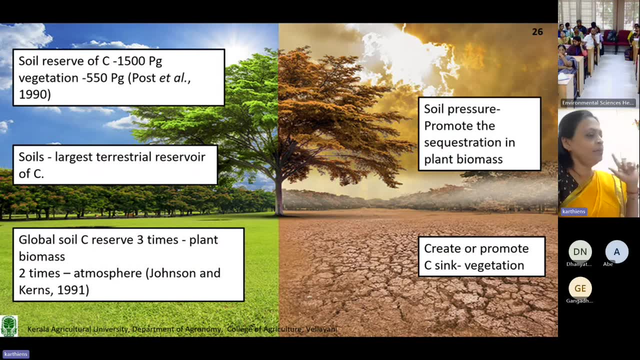 molecular structures, the biochemical structures also. the carbon is sequestered then. so these are some of the data. on the soil reserve carbon: how many petagram of carbon is present? the vegetation: 550 petagram of carbon is present and we can see that because of the, we have to create or promote the carbon sink. 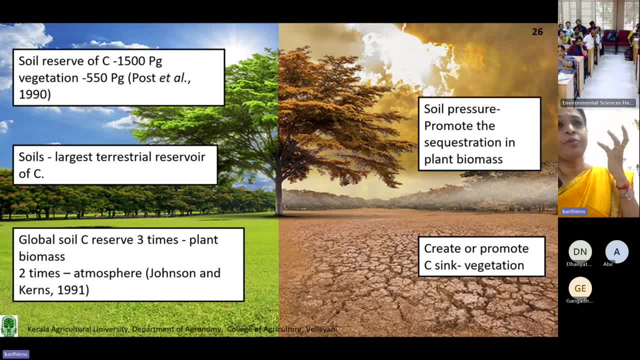 sink is the one in which the carbon is stored. so we have to promote or we have to plant more trees or we have to go for a frustration programs. so in this figure you can see that this is a dry, barren land. here it is a land that is cultivated, where you have freeze and other things, so the carbon that 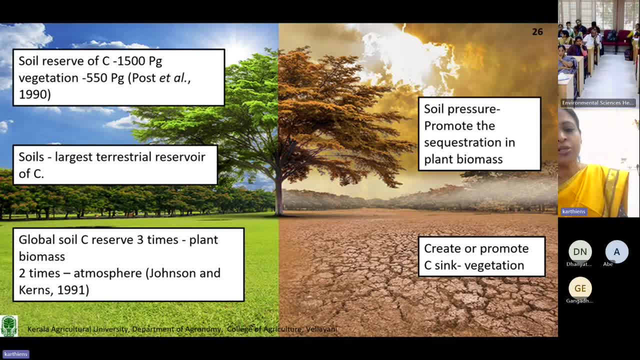 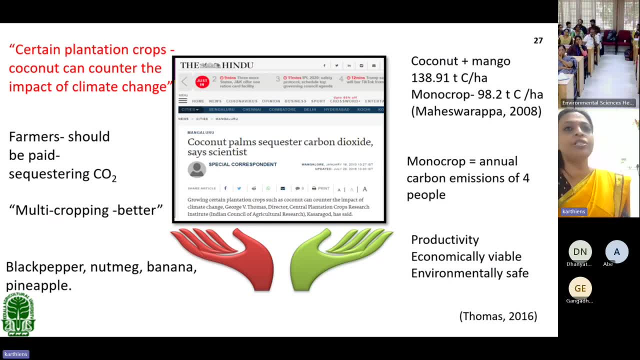 is present in the atmosphere is sequestered in the vegetation. so this is also another important thing which we have to. certain plantation crops can counter the impact of climate change, and one is among the coconut is the most important crop, so coconut can be used as a tree as in a state. 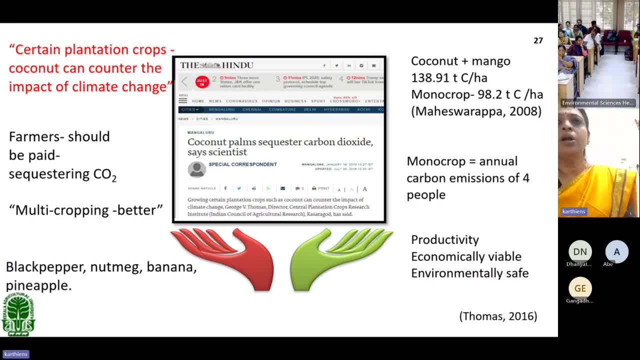 of kerala, which is very small. we have coconut plantations and a lot of coconut can be used for sequestering the carbon in the atmosphere. so either as a monoprop or as an intercrop, you have more options. in the case of coconuts, you can go for a multi-tier system, you can go for a coconut. 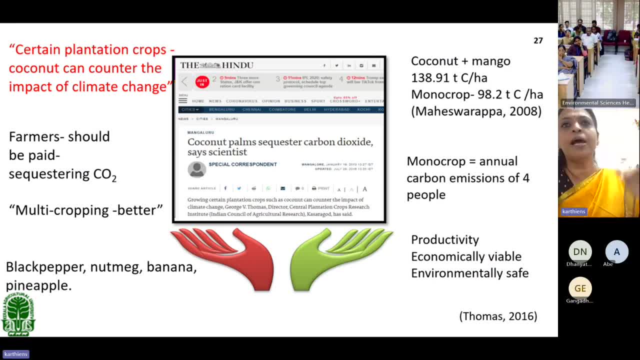 based cropping systems where you can go for intercrops and you can improve the carbon sequestration. so multi-crop cropping is better because at different levels you can grow the crops you might have studied in agronomy courses: multi-tier cropping system at different levels. 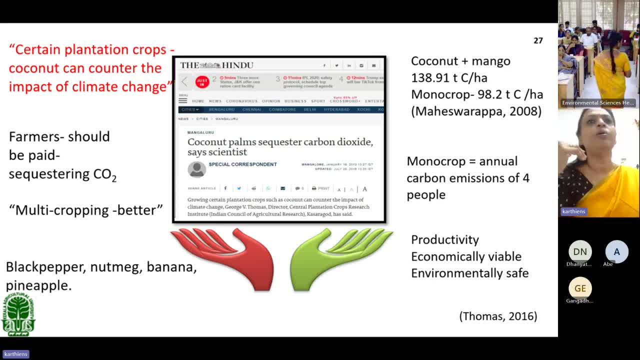 you can grow the crop. nowadays we are going for vertical farming and all where the carbon is sequestered. so, at different levels, the carbon can be fixed by the natural process of horticulture synthesis and the carbon dioxide level can be improved. and on decomposition, these plants will 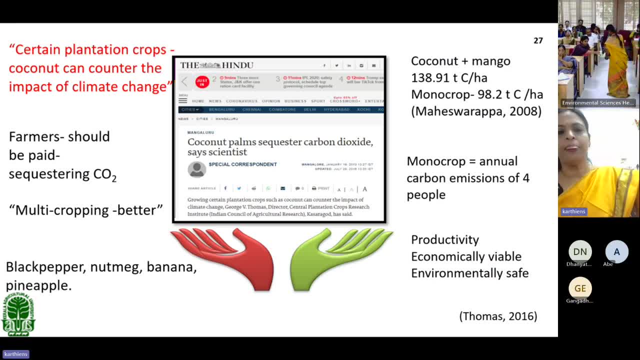 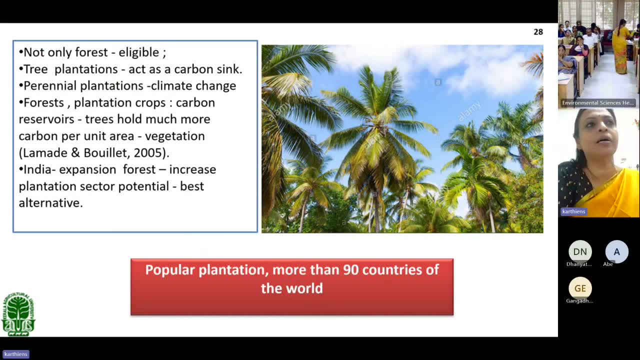 contribute to the soil carbon. so these are the some of the options that can be used. so, forest in the. in the case of forest, if you have forest lands, automatically the carbon will be sequestered and the biomass will be recycled and there will be a natural process of carbon. 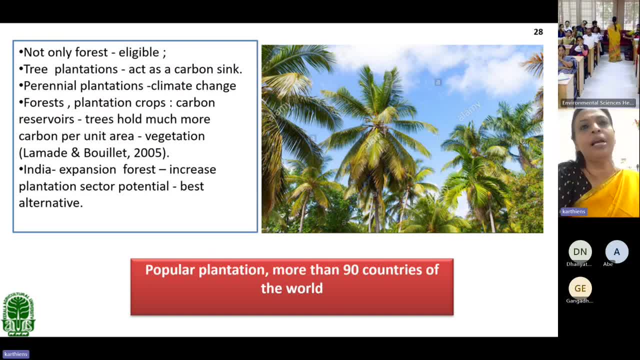 sequestration. but in the case of agricultural or the cultivated land, we can go and plant various pernicious perennial crops, in which the coconut is one most important crop and you can go for, and also teak and other plantation to other long perennial crops can be also grown where the carbon sequestration will. 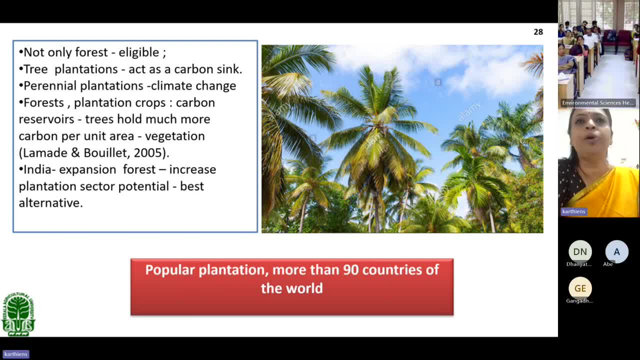 be more. suppose, if you have a barren land, why don't you plant coconut? or why didn't you plant a teak or any perennial crop, so that it can sequester the carbon as well, as it will give you benefit, you to grow it simultaneously further or for greater yield for environment, and not only now with that. 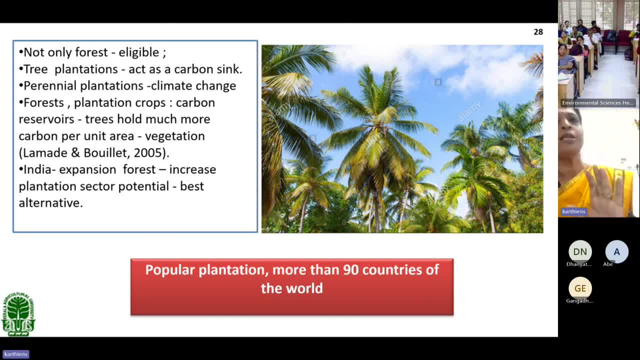 it can grow on the land, but after a long period of time. so they can also. they act as carbon reservoirs and fix that atmospheric carbon. so this is an option that is available. so it is a popular plantation. poplar plantation is a popular plantation. that is more than 90 countries of the 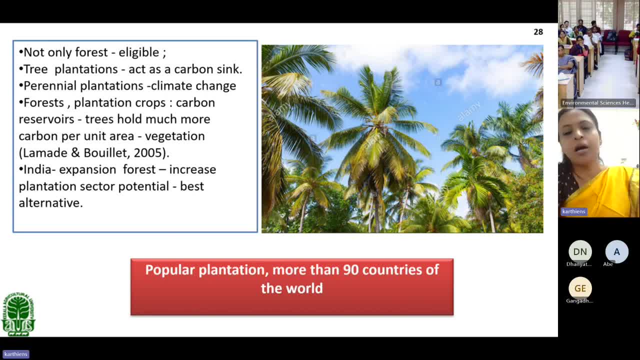 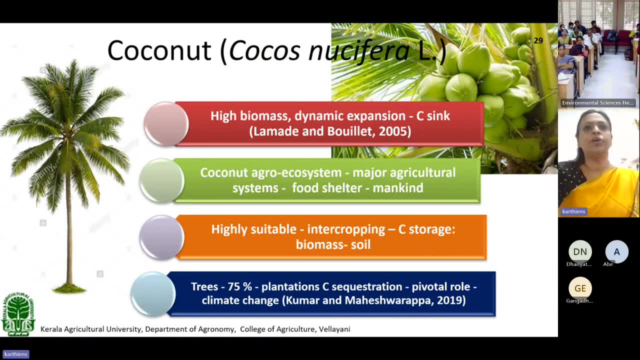 world are growing crocodile and it is. it is a promising crop for fixing the carbon or requesting the carbon, so this is highly suitable. when you go for that coconut, it has you can, you know, you want to, you know the spacing of coconut. so, in the case, what is the spacing of coconut? 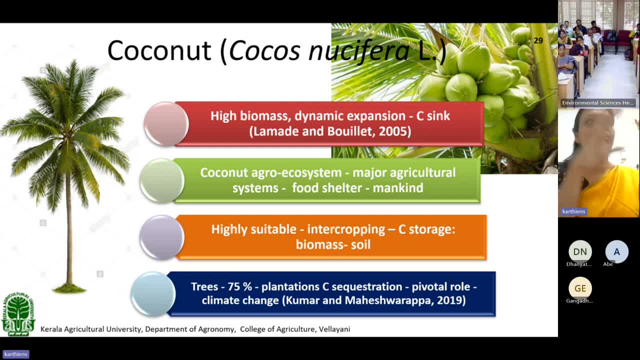 seven into seven, so you have a lot of space in between them and you can also grow intertops like uh at different levels. we can grow and we can um fix the atmospheric carbon also and we can improve the soil carbon status and so many options are available. either you can go as a monocrop or you 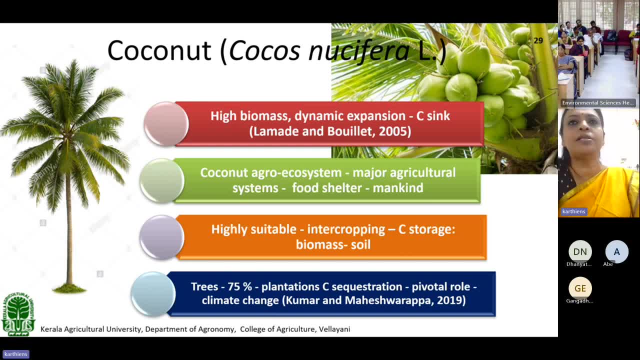 can go as an intercrop or multi-tire system or in the case of homesteads. so homesteads means a small house. a farmer is having a small house. so what is the problem with our? um country means we have small land holdings. we cannot go for extensive cultivation. so in that case, when you have a small 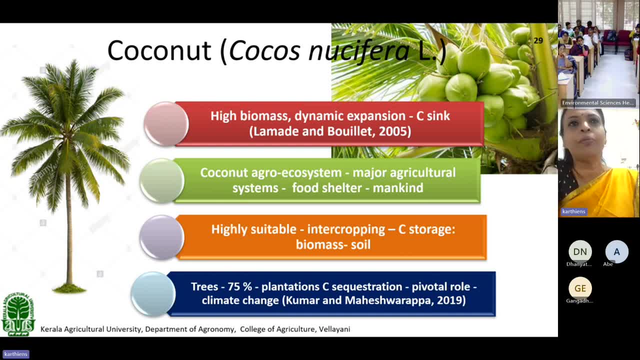 house. with the five cents or ten cents you can plant two to three coconut plants and you can go for uh maintenance of that so that it can also fix the atmospheric carbon. so it is also called as a versatile plant. so it is also called as a versatile plant. so it is also called as a versatile plant. 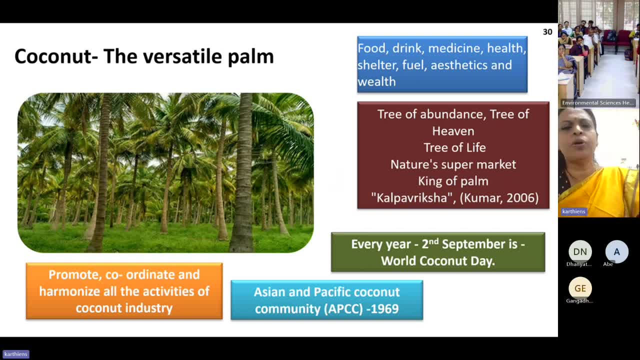 and it is a very important thing, and you know the benefits of coconut also. all these benefits can be also derived. besides, it acts as a very important tool for carbon sequestration. so in the integrated farming system research station at vandrum we have an integrated farming system research station. 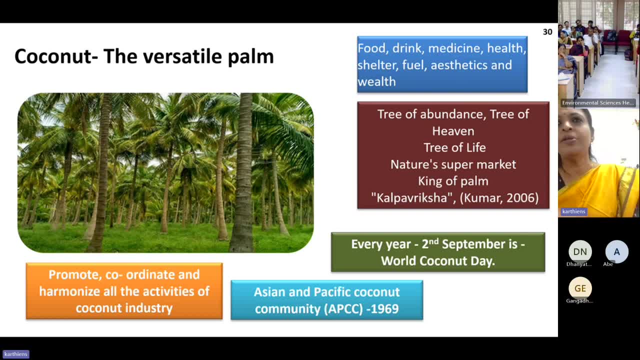 we have tried the carbon sequestration still now. now it's a even now we have a project. so the carbon neutral agriculture. it has been evaluated for the different cropping systems- rice based cropping system, coconut based cropping system, banana based cropping system- and it was found to be that this coconut based cropping system is found. 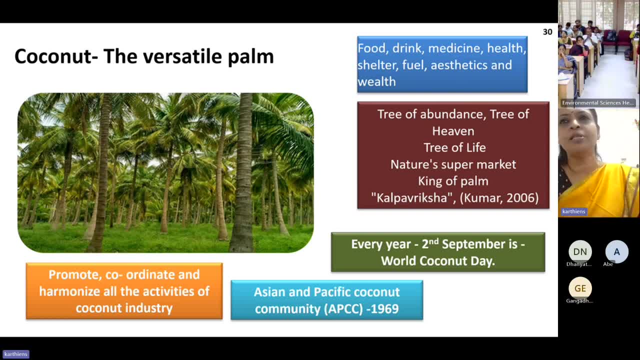 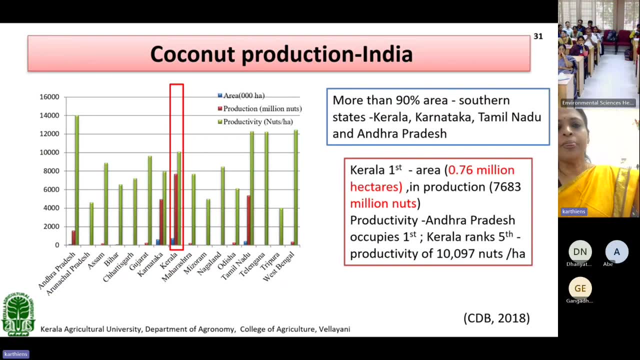 to be the most best and reported highest values for the carbon sequestered from the atmosphere. then the rice, the base cropping system, as well as the banana based cropping system. so so this is the data about the coconut and opportunities. either we can go for intercropping or monocropping, or 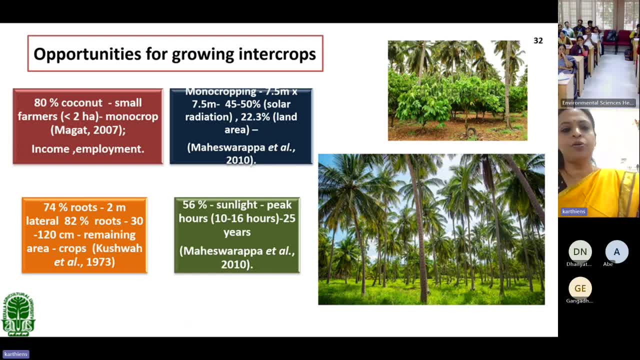 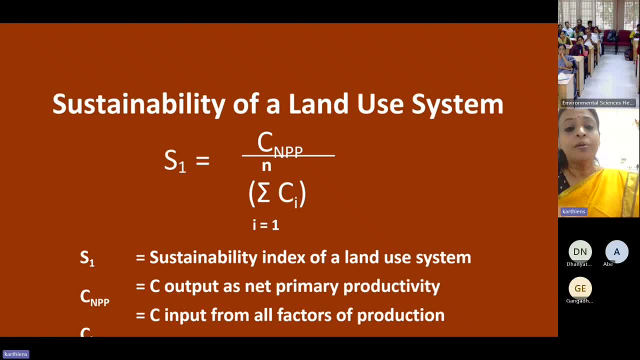 we can also go for as a single crop also. this can be also grown then. sustainability of the land use: you can work out the sustainability of the land use system by taking into account the carbon. so you can see the form. instability of the land use system. so sustainably. index of the land use system. when? 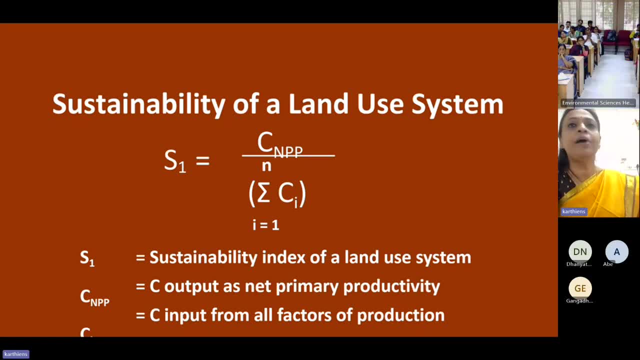 you are using a. when you are evaluating a system, we have to evaluate whether it is sustainable or not and see output as a net primary productivity and the c input. that is why the carbon is very important. c output and c input should be taken into account and we can work out the. 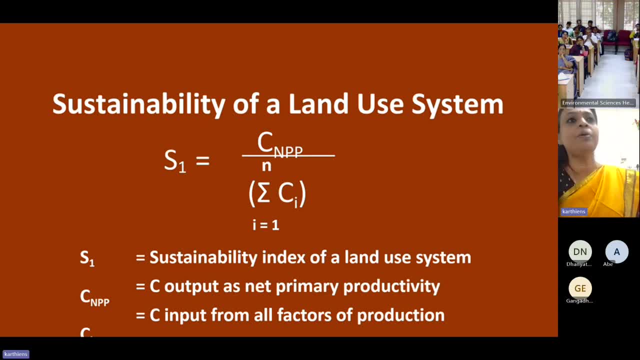 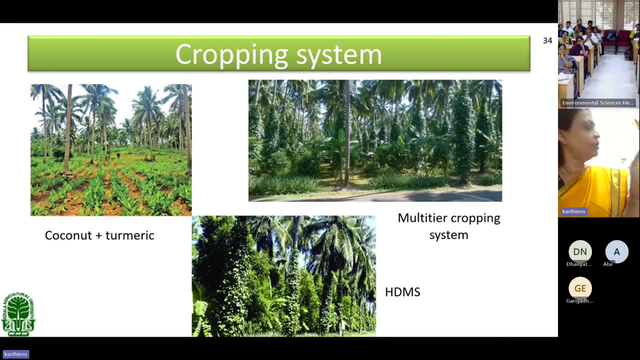 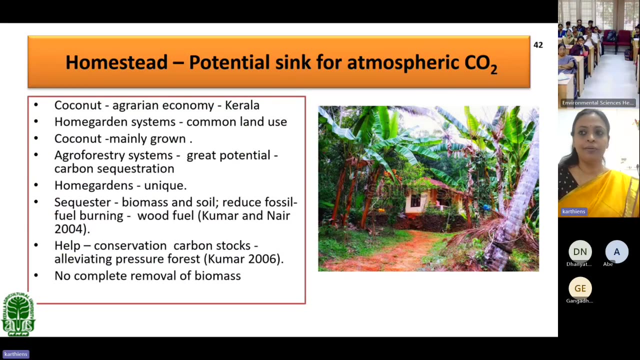 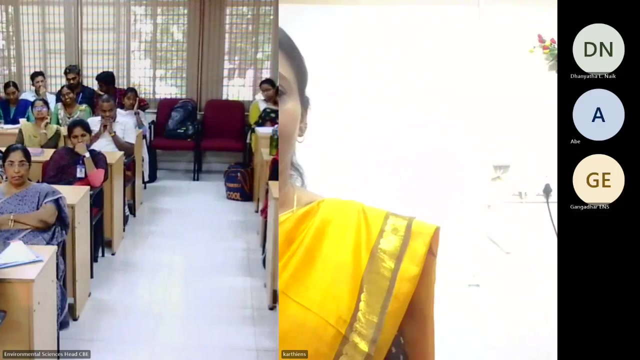 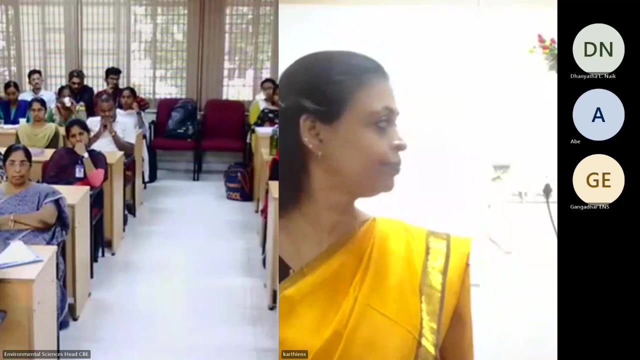 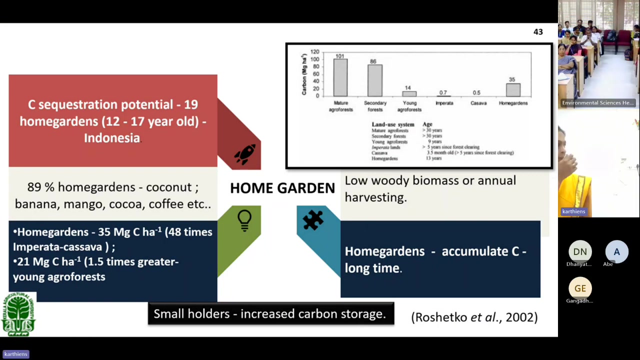 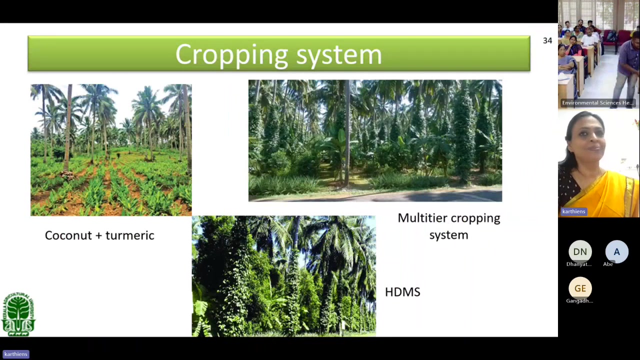 sustainability of the system. we can work out whether the system is sustainable, whether it can persist or not, and that can be worked out by using this, calculating this index. then these are some of the systems which are available. close it will close it the tension. this is so, in the case of within 10 to 15 minutes, i'll continue to stop it. so coconut and turmeric, and 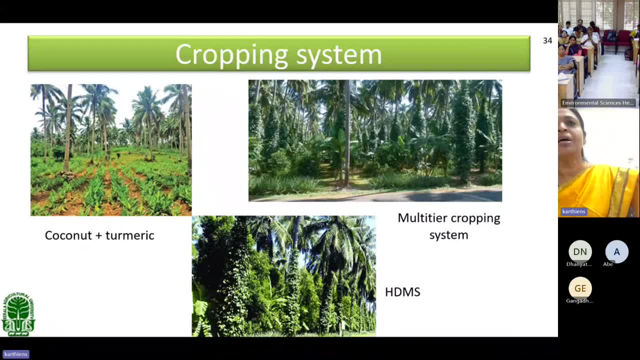 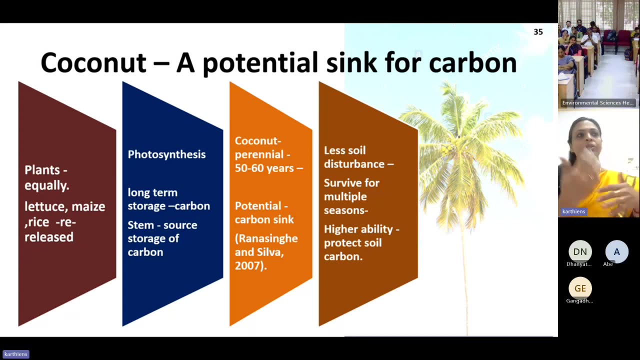 that is one option that is available. then we have the multi-tier cropping system and high density multiple planting. hdmp is also another option that is available where we can go for, uh, i think so. these are some of the important things. why, uh, we are going for coconut and why? what are the various? 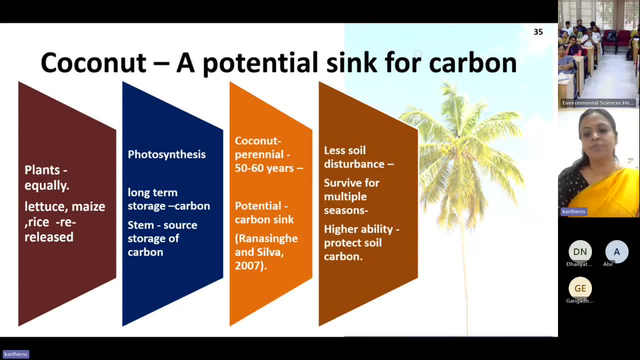 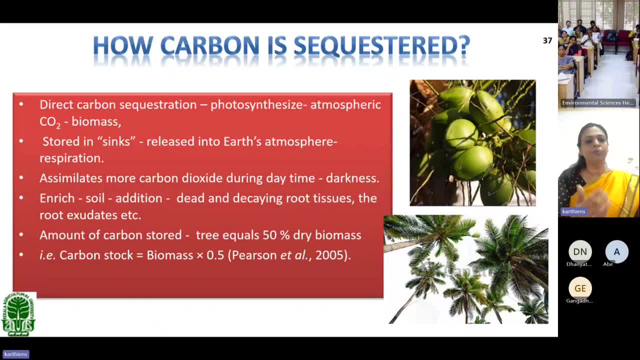 uh land use systems, and we can also work out the sustainability of the system, whether it is sustainable or not. like that we can work out, then, how the carbon is sequestered. so the carbon is sequestered either in the form- of that already we have seen- either in the form of oceanic or 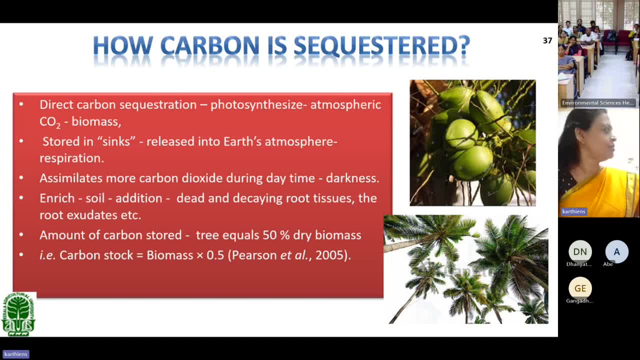 terrestrial or aquatic, or by the microorganisms- and there are so many mechanisms- or by the plants and after the decomposition that will add to the soil, that will add to the various fractions of the carbon in the soil and improve the carbon content of the soil. so that is also another. 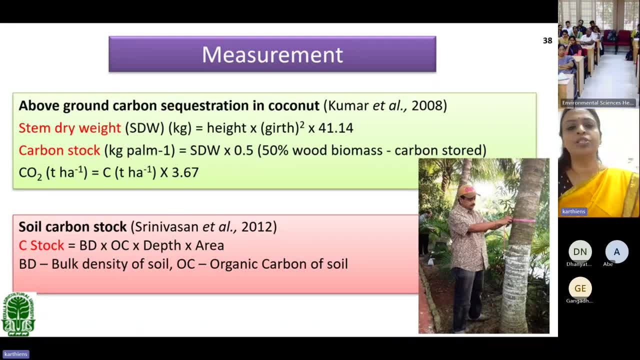 mechanism by which so we can also calculate the soil carbon stock by using the formula bulk density into organic carbon into depth, into area, so by that we can work out the whether the soil is sustainable or not. if the soil organic soil carbon stock is more, then we can say the system is very. 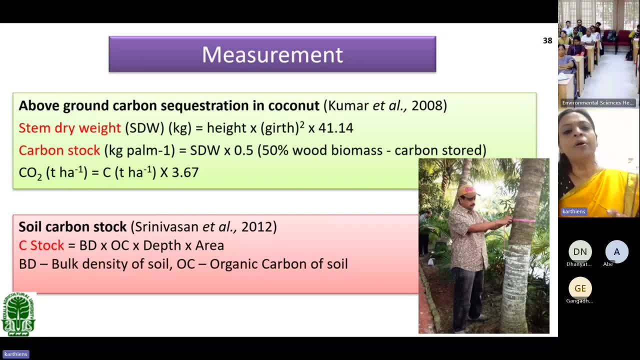 uh, sustainable and also we can also work out the above ground, carbon sequestration. so that was calculated. so in the integrated farming system research station we have calculated the carbon sequestration in the coconut palms by using this formula. that is a swe, that is height into girth. 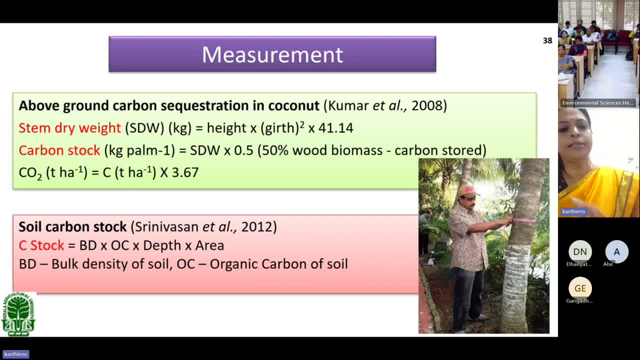 into forty one point one four. so this is another important uh thing, and also we can also find out what is the carbon stock that is requested per uh palm per year. that can be also calculated. so these are some of the important things. then equipments: we have an equipment that. 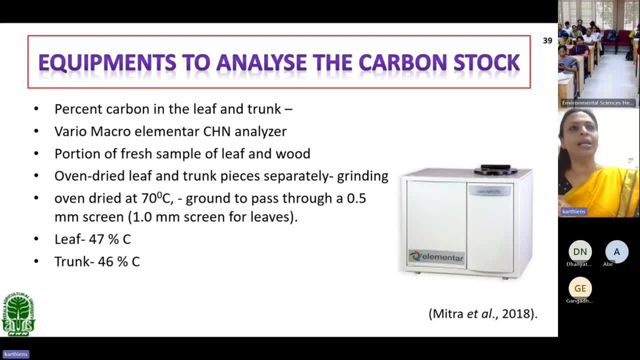 is macro elemental chn analyzer. so elemental analyzer, chn, carbon hydrogen, that is, carbon hydrogen and nitrogen analyzer that is available and by using this we can find out what is the elemental content. so we have to over dry the soil and pass through it and now we can find out. 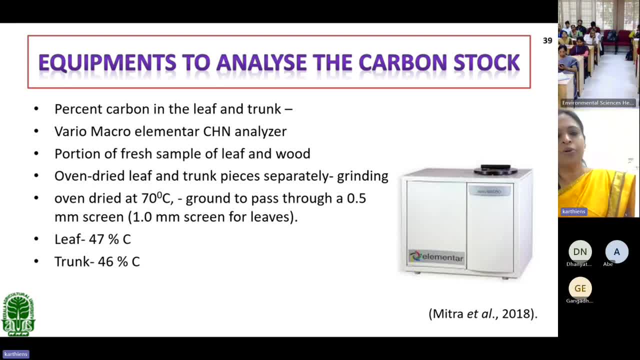 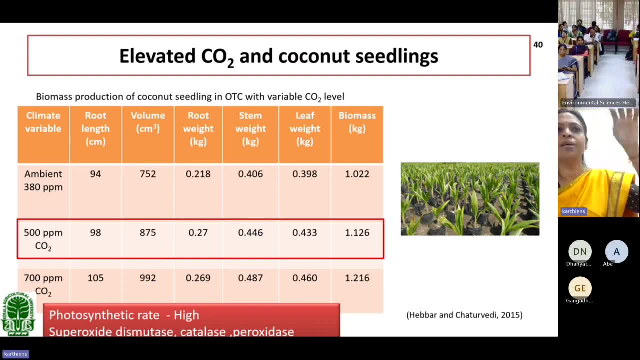 what is the organic carbon content of that particular fraction? that can be also found out then elevated carbon dioxide and coconut ceiling. when we in carbon dioxide chambers we have given different levels of carbon dioxide pressure and at higher, it was found out that at 500 ppm of carbon 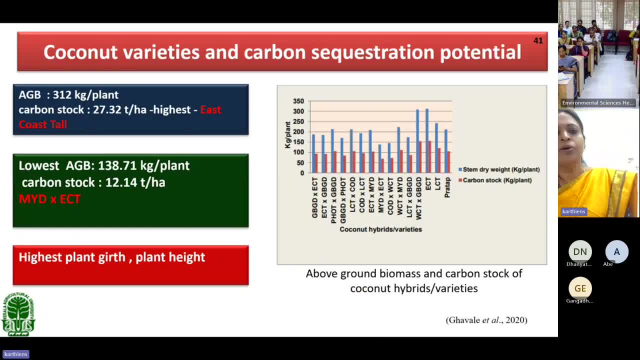 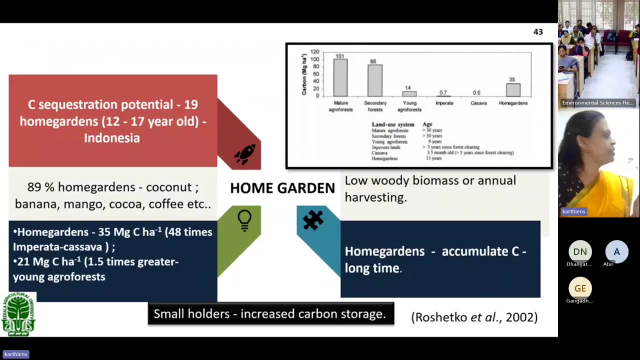 dioxide. the performance of coconuts, or ceilings, were found to be high, and also the varietal some varieties are very good for within the coconut itself. there's some varieties are very good for sequestration. then, as when we see that the carbon sequestration potential of 19 home gardens 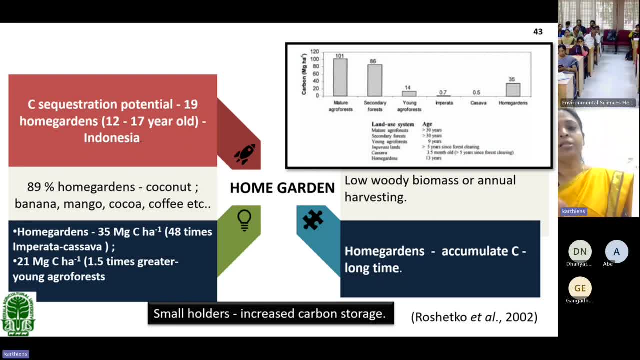 were taken in indonesia. the data is also provided and you can see that the plants, the gardens with coconut plantations- as coconut has major crop as the intercropper or main tropper, that is found to be much higher in sequestering the carbon compared to the other other plantations. and we can also go. 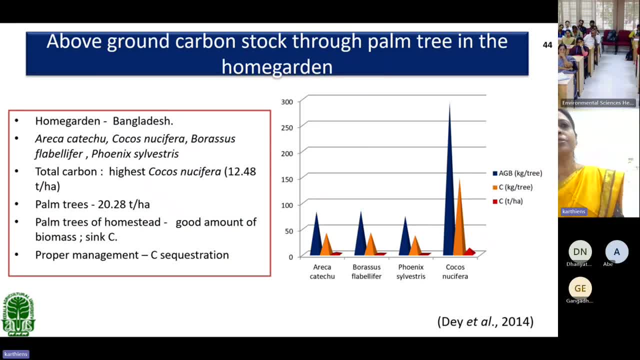 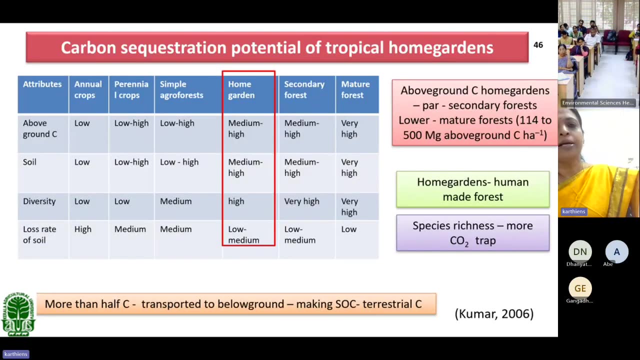 for other uh. we can also go for other related palms, reconnect and also other types of palms instead of coconut in order to fix the atmospheric carbon dioxide, and we can see that nearly twenty to twenty two or twenty eight tonnes of carbon can be fixed per year per hectare and 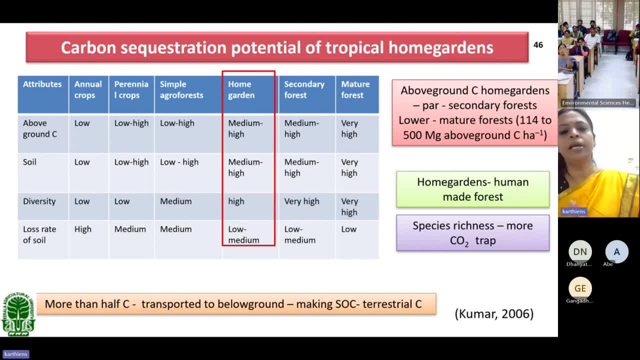 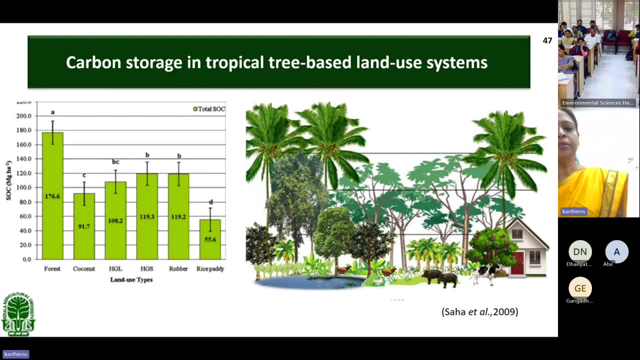 the home garden. also, we can go for the typical coconut and and we can see that the amount of biodiversity, as well as the soil, organic carbon, as well as the soil loss rate will be reduced when we go for this coconut plantation. and this is the data on. 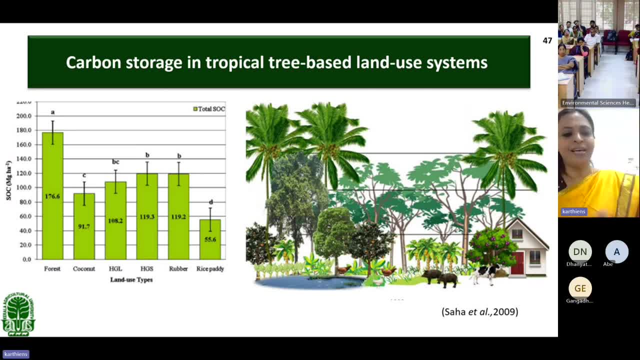 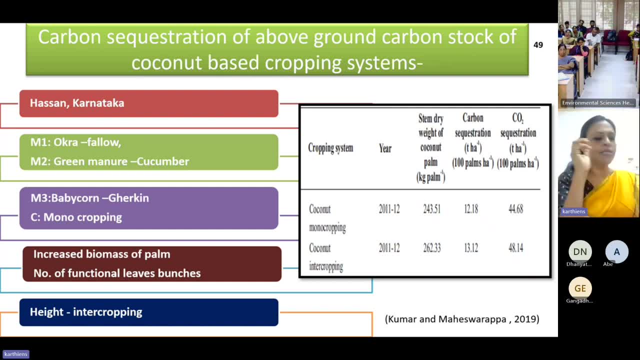 the soil, organic carbon in the land use type and it is not coming anyway. so cropping system and the carbon sequestered. we can see that in karnataka the okra and fallow green manure, cucumber and so many combinations have been tried. so coconut mono cropping and coconut. 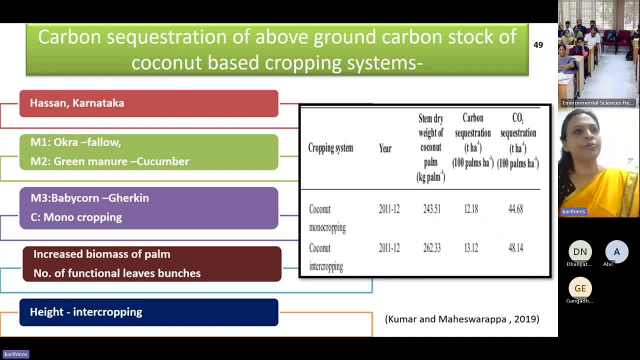 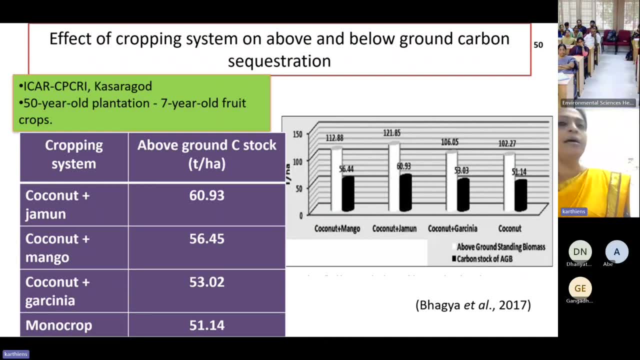 intercropping. so always we suggest a coconut intercropping in order to sequester the more amount of carbon from the atmosphere, and coconut plus jamun, coconut plus mango, coconut plus garciana garciana, kodambuli, that is, that can be used, and monocrop of coconut, that can be also recommended. 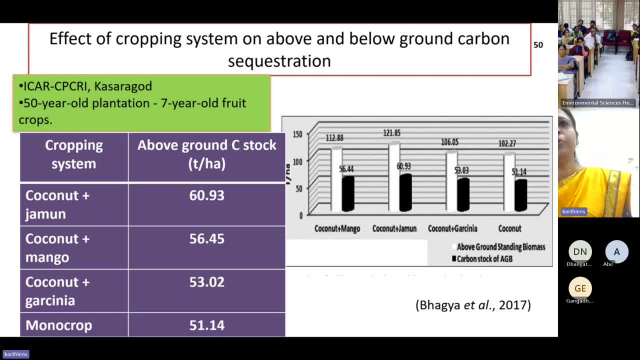 for sequestering the carbon. so, instead of monocropping, if you go for an intercrop or a multi-tier cropping system, you can. this was an important work by icr, cpcra, casar voda, central plantation crop research institute. you can see that the carbon sequestered and the carbon sequestered and the carbon sequestered. 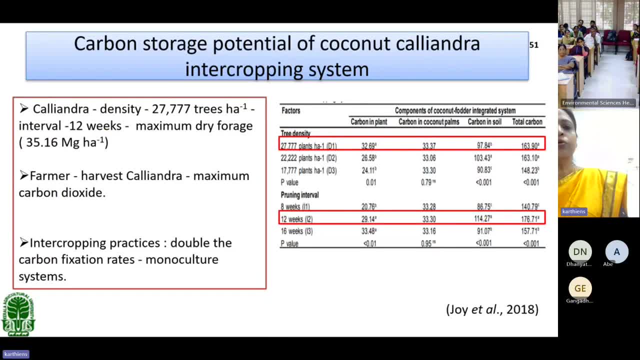 they have found out. then here also in the carbon storage potential of coconut caliandra in intercropping system was also worked out and we can see that the harvest caliandra maximum carbon dioxide was sequestered with that and the intercropping practices was also found. 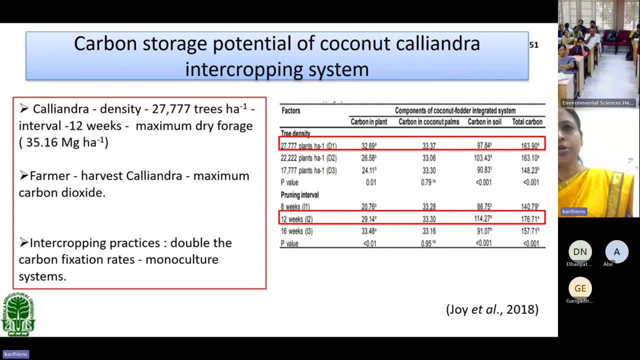 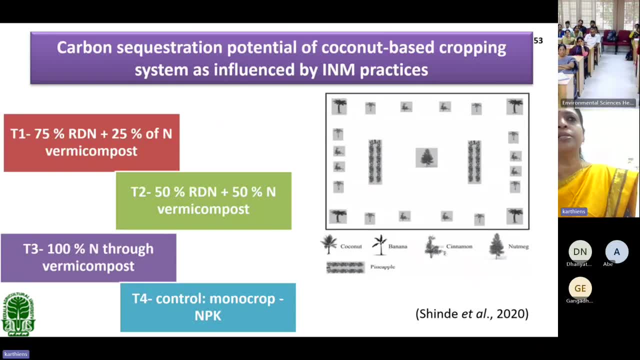 out and we can say that no intercropping, no tillage was carried out in these operations. then in the case of nutrient management and carbon sequestration, we have this organic matter addition and organic uh, all these things integrated nutrient management. you know, where 75 percentage of the nutrient is substituted with the uh, the 25 is substituted with the organic. 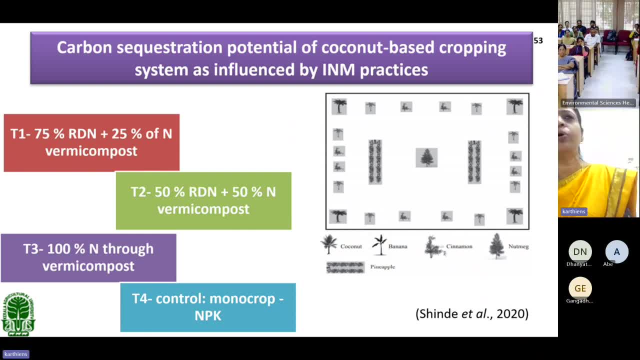 manure also. so always uh. when we integrate the nutrient with the organic and inorganic sources, we can sequester maximum amount of carbon and instead of going for 100 percentage of inorganical whatever when we have a lot of bio waste, like a farm waste and farm. 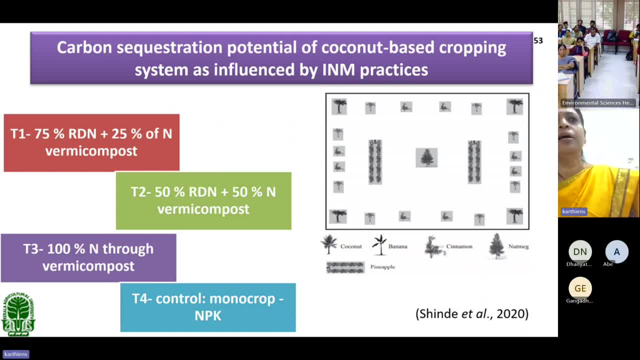 residues are there, you can resort to the composting and other techniques in order to avoid the release of carbon dioxide into the atmosphere and fix it so that you can use these menus as well, as this can be applied to the soil for improving the carbon status. 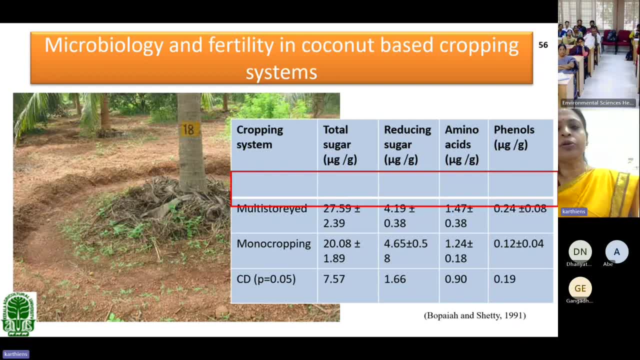 So this is microbiology, When you work with the microbiology, and fertility also, and the microbial population was also found to be high in the coconut-based cropping system when we found out that, because it is directly related to carbon status also, So always a direct positive relationship with the carbon. 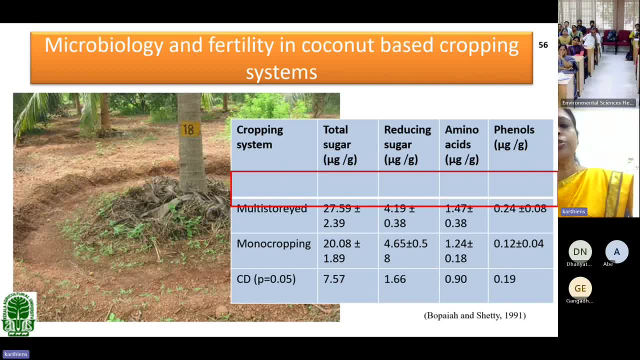 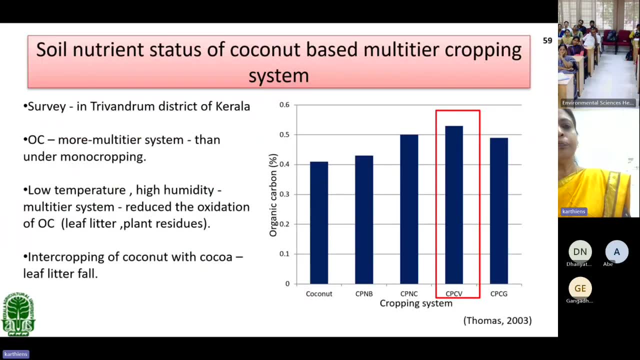 And another important parameter is all these total sugar reducing sugar, amino acids. all the quality parameters were also found to be increased. And then multi-tier cropping system, When you go for the survey was carried out in Trivandrum district and we found out that organic carbon was found to be most highest in the case of the multi-tier system. 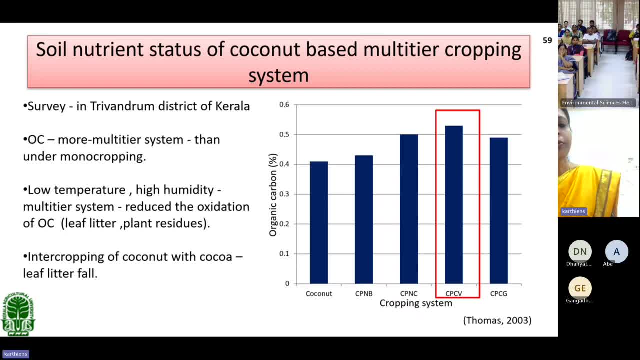 than under the monocropping system. And these are some of the Well. the intercropping of the coconut with cocoa. So in Wayanad district we have intercropping of coconut with the coffee. Coffee plantation is the most important thing where the land is completely covered up. 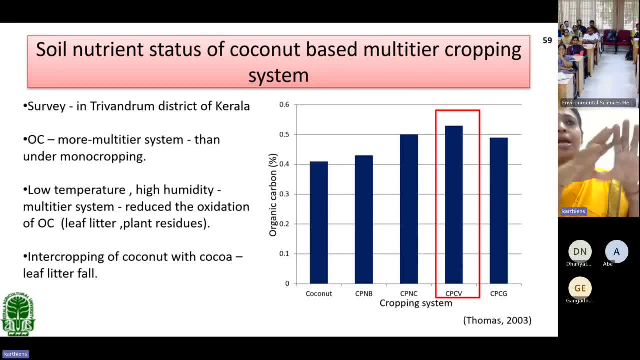 I mean no land is left to fallow and everything is covered And the land, the integral, the entry area between the trees also not left free so that everything is covered with a canopy. So the microbial population as well as the organic carbon, everything is high in those soils. 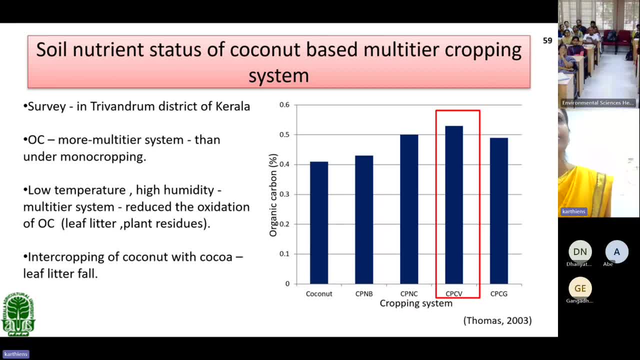 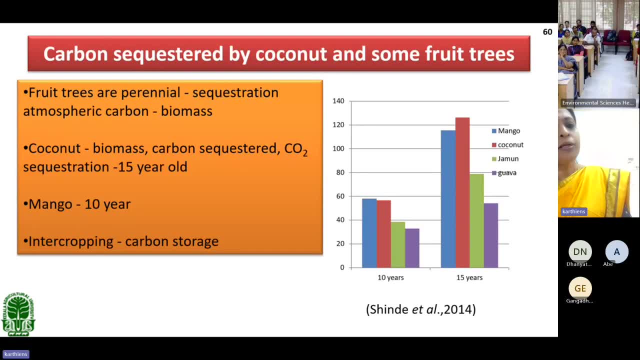 The Wayanad soils. So when compared to the other soils also, That one of the reason for that is the amount of carbon sequestered is high when compared to the other cropping systems. And it was also found that when you take coconut it takes 15 years more. 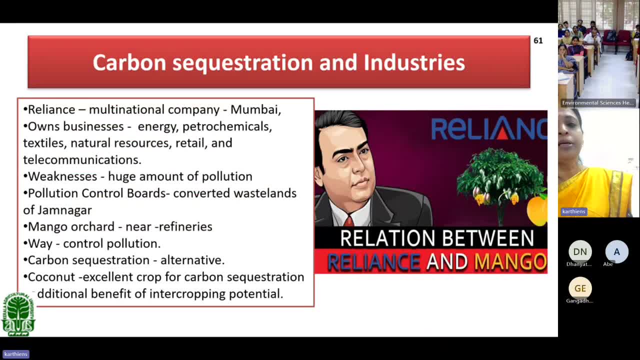 and mango 10 years. it will sequester the highest amount of carbon And industries also. we can see that industries also will contribute to the carbon contributions. So, as pointed out, industries have its own merits and demerits And even though 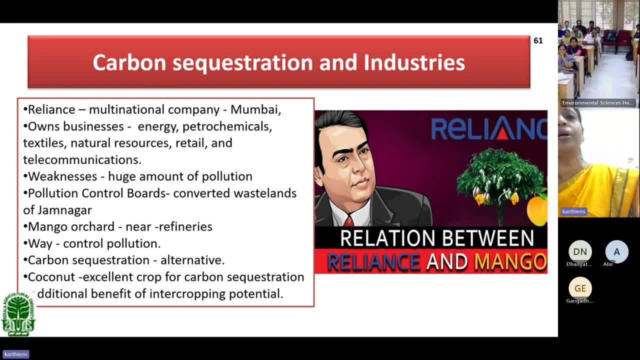 Even though they give a generation employment and also contribute to the economy of a country. some of the problems are there. They release carbon dioxide, as told, heavy metals and all these things will be released into the ecosystem. All these problems will be there. 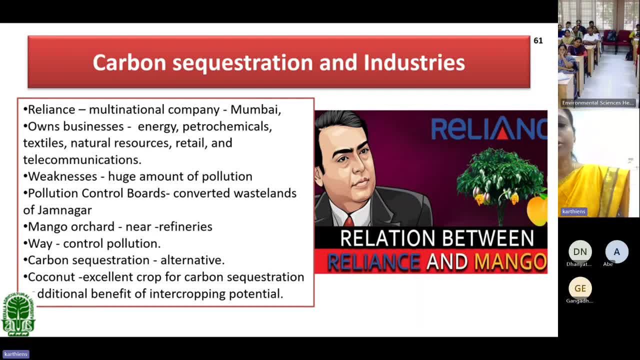 So Pollution Control Board is also giving so many regulations and rules in order to especially the Reliance Control, And they are also promoting some plantations in some of the areas in order to fix the carbon dioxide. So it is one of the activity of the Reliance Company. 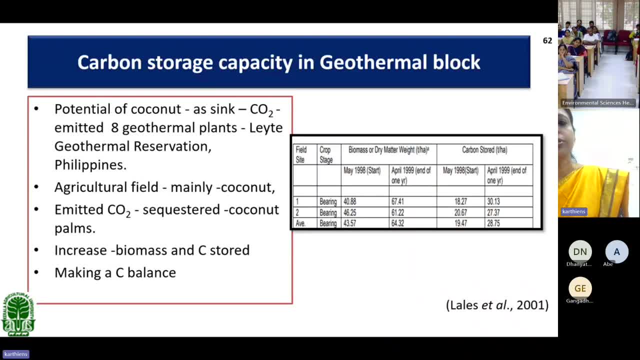 To fix the carbon dioxide that is released by their industries, Then Philippines- Philippines also won geothermal reservations. So whatever industries they are doing, they are doing the carbon sequestration activities- Either growing plantations or any of the trees- in order to sequester the carbon that is present in the atmosphere. 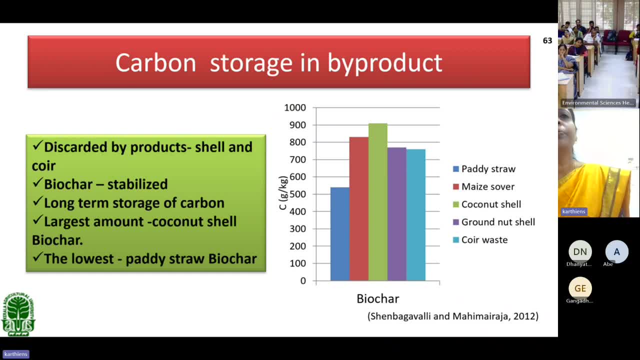 Then we can also buy products. So when we use this coconut as the agent for carbon sequestration, we can also buy products. prepare biochar. biochar is a very good um source of carbon that contains recalcitrant carbon. when you apply the coconut biochar carbon, when you apply to the soil, it won't. it won't be decomposed. 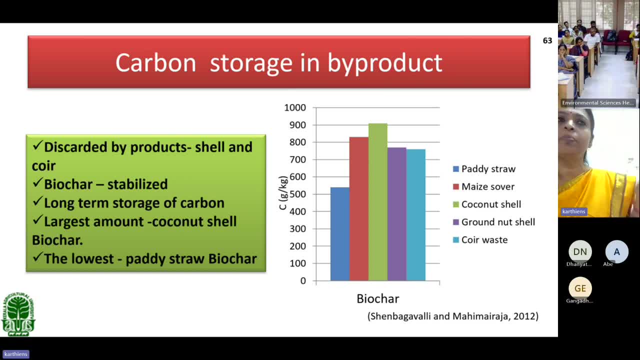 it will be retained in the soil and the recalcitrant fraction will be more when compared to the other fraction. so, uh, coconut has can be converted into biochar, and the temperature and everything can be. you know, biochar is a method that is prepared by pyrolytic method. in the absence, 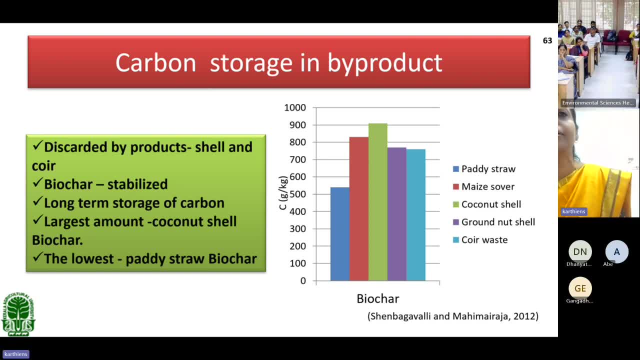 of oxygen, the controlled oxygen content. so biochar is a very important one that contributes to the carbon fraction, especially to the recalcitrant carbon fraction, and also, in the case of paddy straw, biochar and all these things, when you come, convert these byproducts as told. 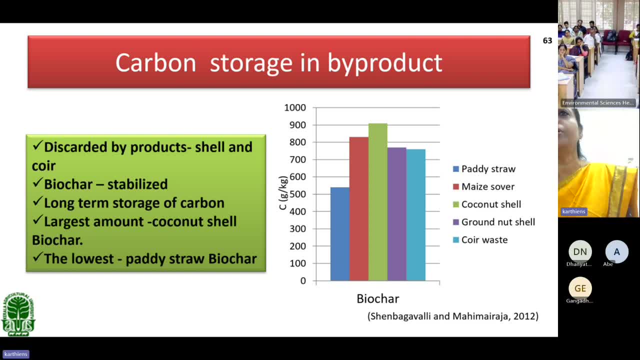 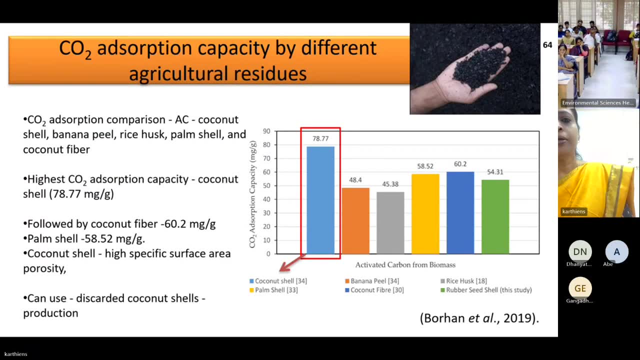 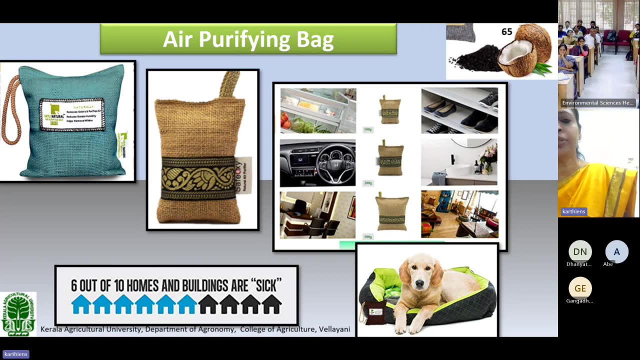 guinea grass is converted into biochar and that is applied, that will improve the carbon fraction in the soil. that is also one of the method to sequester the carbon and a different. so these are some of the air purifying bags are also available as a product. so these are all the products which are 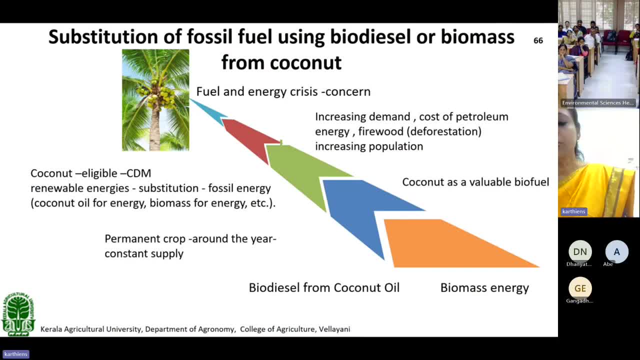 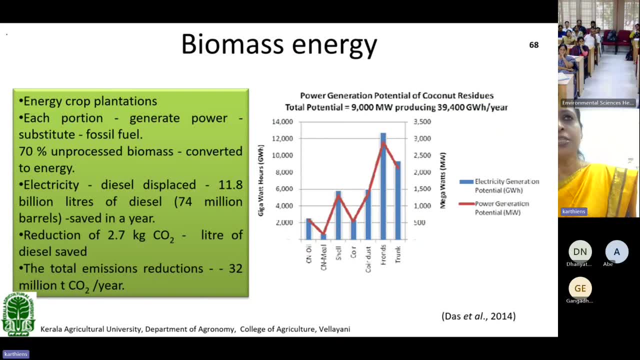 which can be used for making us. so from the coconut we can also get the biodiesel and bio fuels and other things, and biomass. energy is also created from the coconut. that can be used for substitute for the electricity, along with that other, so the total emission reduction will be 32. 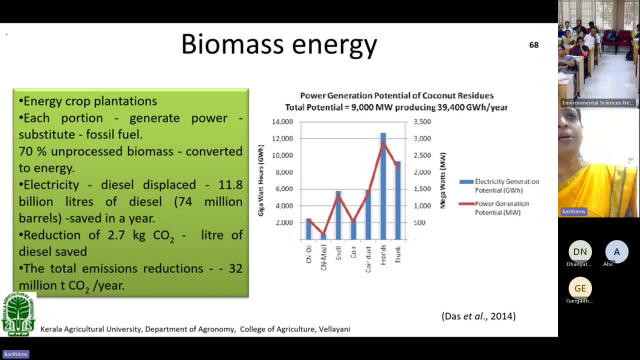 million tons of carbon dioxide per year, that is, can that can be reduced per year? so what is carbon credit to? carbon credit is a limit that is fixed by the each company, that is, each country. how much of carbon that can be released into the atmosphere. that is a ceiling for each and every country. 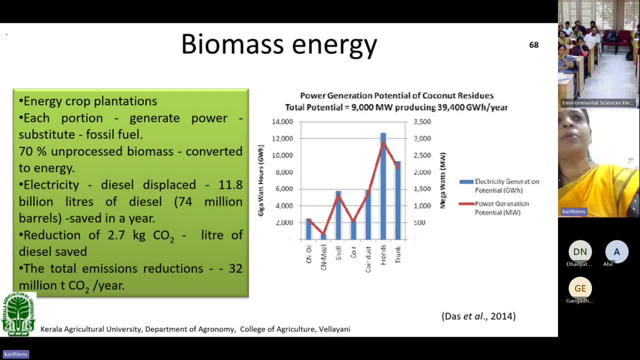 suppose you are not using that ceiling, you can sell your carbon credit to some other country, so that is called as a carbon trade. so carbon credit and carbon trade and all you will be very much thorough. so all these things are based on the carbon sequestration and also considering taking into consideration the carbon. that is, that 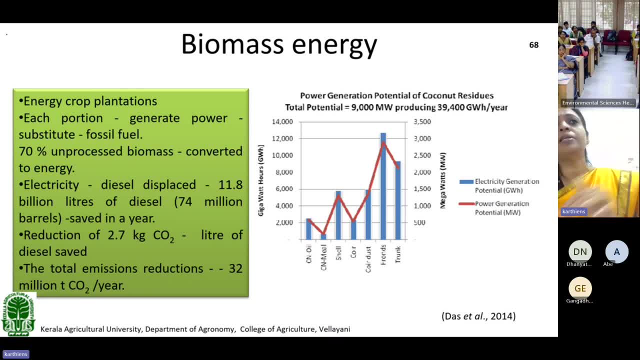 is to be present in the atmosphere. so carbon credit is the limit that is fixed by the countries where for the amount of carbon that is released, that is, that can be released per year. so if you are saving your carbon by these methods, if you're seeing a carbon release, you can sell it to your 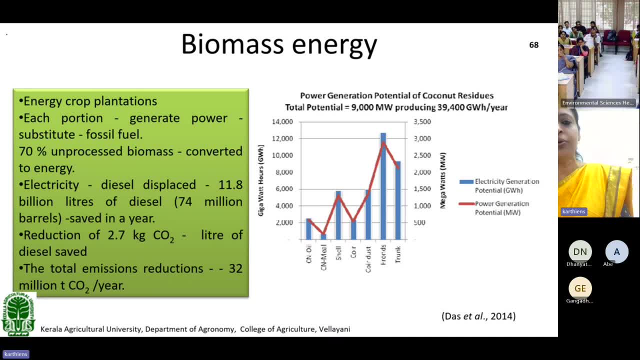 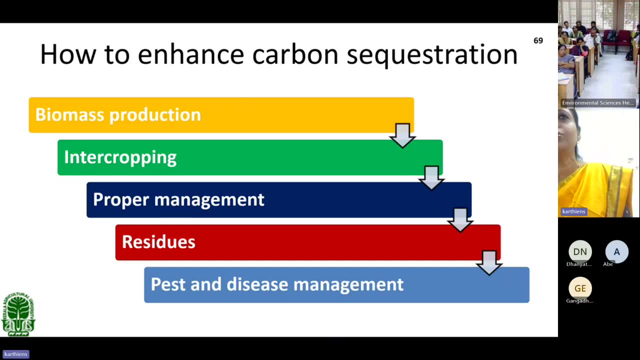 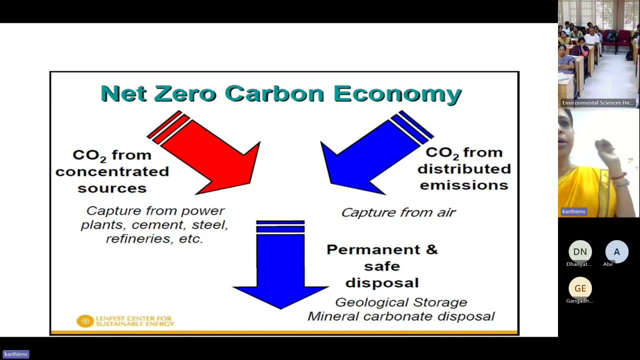 other country and earn money from the other country, which is called as carbon trade also. so biomass production, intercropping management, residues, pest and disease management, don't apply so much of chemicals that can also, so we can achieve for a net zero carbon economy. net zero carbon economy, that is. 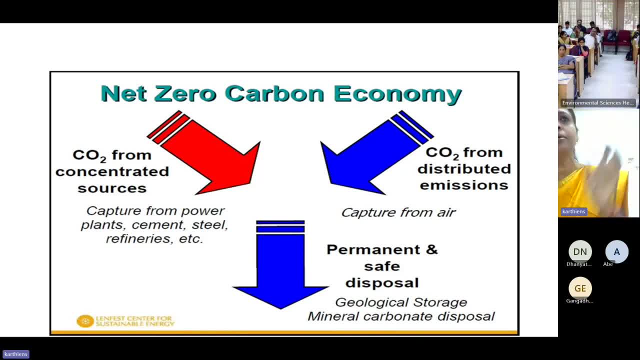 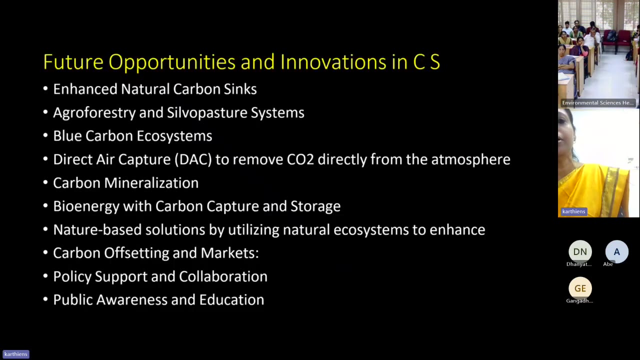 we can uh ascertain, we can attain carbon neutral uh at a particular point, not only in immediately, but after a few years. when we follow all these guidelines uh- carbon dioxide from the concentrated sources, from the distributed emissions, and also safe disposal- all these things we follow all these protocols very um uh strictly, we can achieve this so future opportunities and innovations. 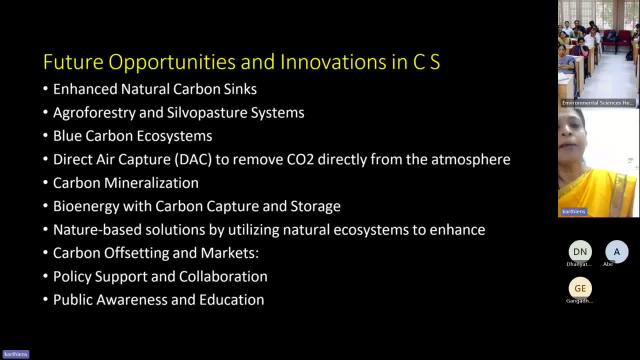 in carbon sequestration. enhanced natural carbon sink, agroforestry and the silvy pasture systems. by this we can sequester carbon, blue carbon ecosystems. that is the carbon fixing by the oceans. direct air capture to remove carbon dioxide directly from the atmosphere. provisions for direct air capture: carbon mineralization. 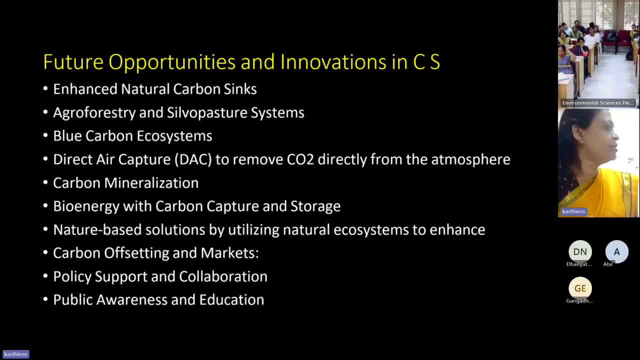 by the oceans, direct air capture, carbon mineralization, the bioenergy with carbon capture and storage, natural based solutions by utilizing natural ecosystems to enhance carbon offsetting. and markets and policy and support. policy support and collaboration is very important and public awareness and education. that is the most important public awareness and important education you have. 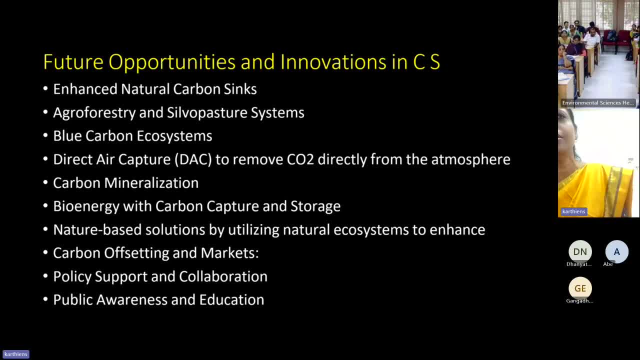 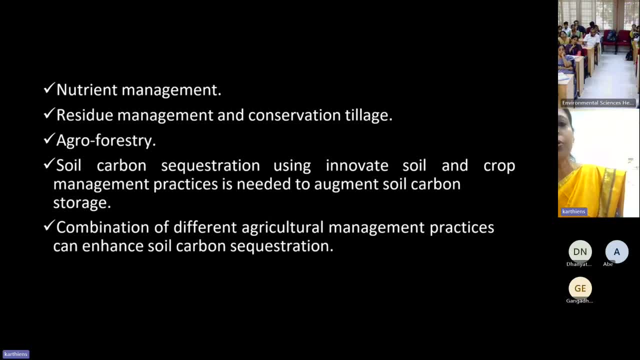 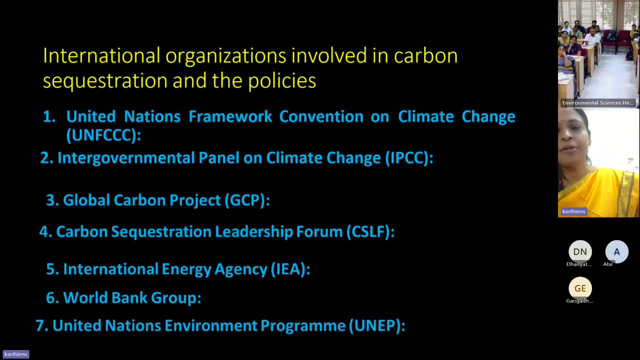 to educate the farmers, farming community about the carbon neutral and the importance of carbon. the nutrient management, residue and management residue management, agroforestry- all these can be also followed. then these are the important organizations related, that is, unfccc, then intergovernmental panel on climate change, then global carbon project, then carbon sequestration.